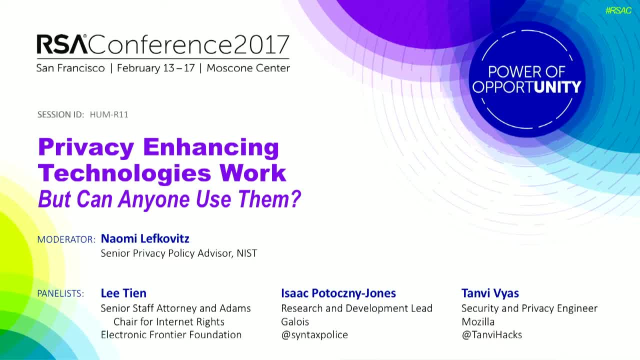 tries to safeguard it from hackers, internal threats, government subpoenas, etc. And it offers features to users to work with. Okay, So privacy-enhancing technologies are tools that allow users to either increase or decrease their privacy at a given moment so that they can improve their online privacy And the 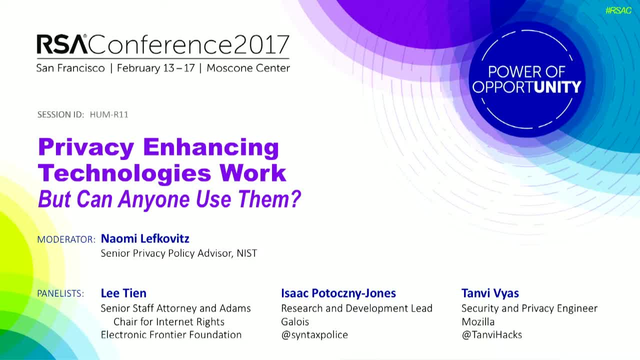 privacy-enhancing technology I work on the most is Firefox, and we provide tools like tracking protection, cookie-blocking options, containers that help segregate multiple identities online, and privacy features like that. Isaac, My name is Isaac, and when I think about privacy-enhancing technology, I like to focus. 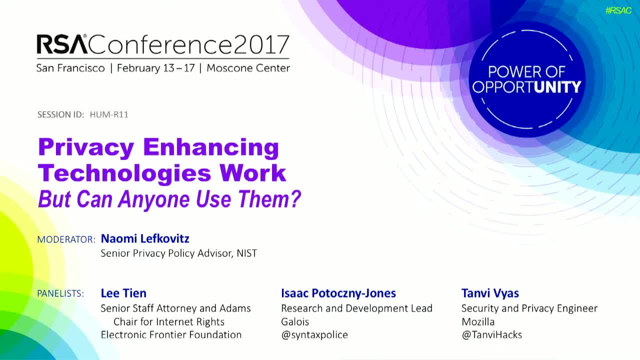 on the kind of everyday decisions we programmers or software developers make when we add features to systems that are not otherwise necessarily focused on privacy. So almost every system out there is collecting information about users, and they make decisions about how that information is handled. 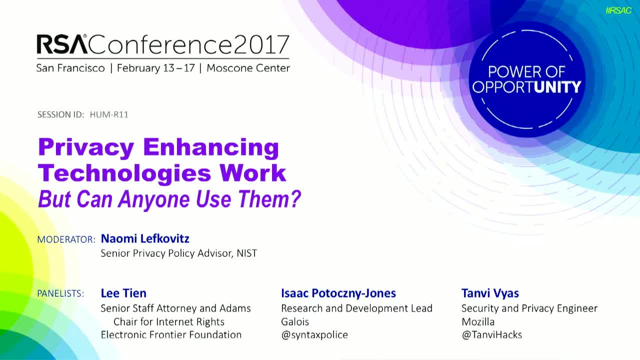 Okay, So what kind of data is handled, exposed to users, what kind of transparency they have, what kind of consent they have about how that data is managed and shared with third parties, And so those kind of everyday decisions really have, I think, the broadest impact on privacy. 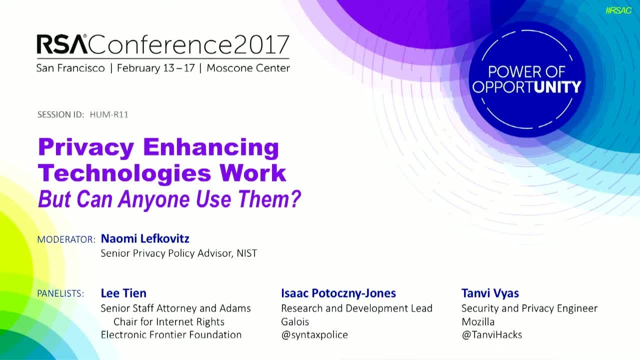 in technology. So our work is in cybersecurity and encryption, particularly focused on building tools for programmers themselves, Because for all of us, security, encryption, privacy are hard, and for programmers it's actually pretty hard too. The same educational challenges for normal people are there for 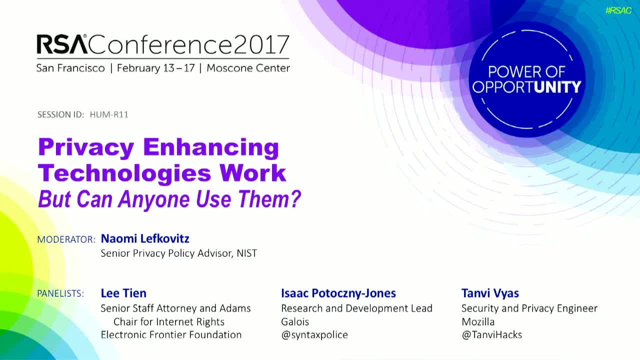 developers when they're actually building those tools into their systems. So I'm Lee Tian with the Electronic Frontier Foundation and I'm an attorney- I'm not a technical person, So naturally my perspective on privacy-enhancing technologies is somewhat crude. You know, I think of a door as a privacy-enhancing technology, One of our most popular giveaways. 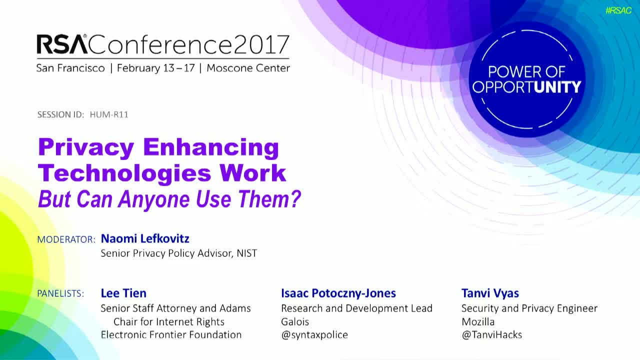 at EFF is a strip of stickers that you can put over the camera on your laptop. That is a privacy-enhancing technology. We also work on Let's Encrypt HTTPS Everywhere- Privacy Badger at EFF, and these are all tools that are free. that are also privacy-enhancing technologies, although in rather different. 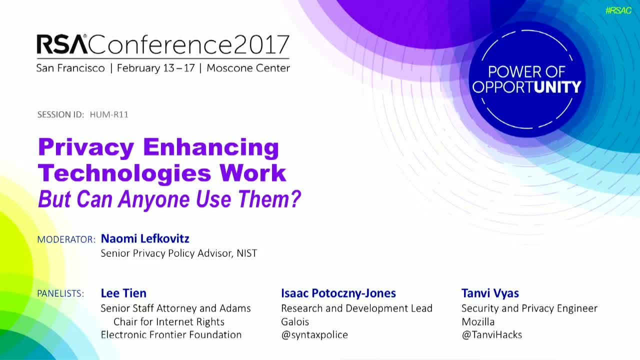 ways right. One of the most basic ways is to block collection, to have control over what information is actually collected about you, But sometimes you need to know that there's even any collection going on before you can do that. So things like our privacy. 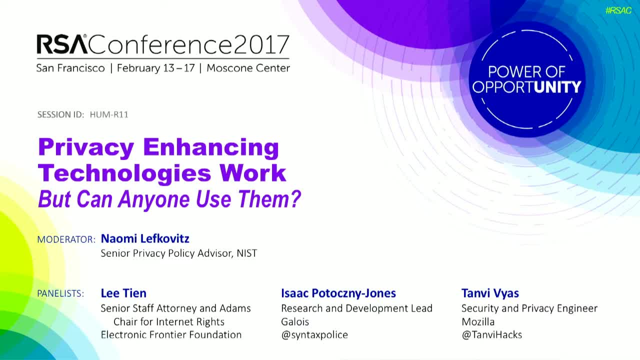 badger tool. it's not an ad blocker, but what it does is it allows you to see what kind of third-party code is on a website that you're visiting, so that I can go to the Washington Post page and it will tell me that there are 60 different other domains than the one. 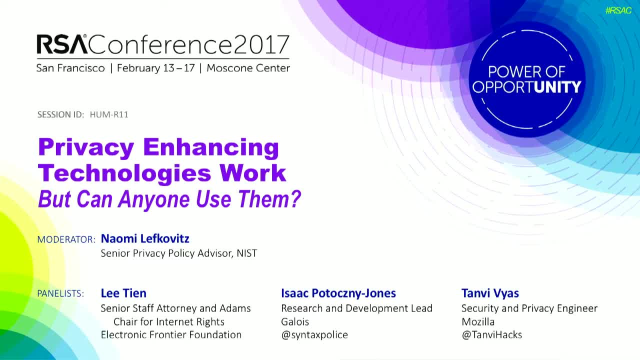 that I think I'm connecting with, and then it gives me the ability to block off those domains. But if I didn't know that there was third-party tracking code, How would I be able to do anything about it? Similarly, Let's Encrypt is an insert bot. 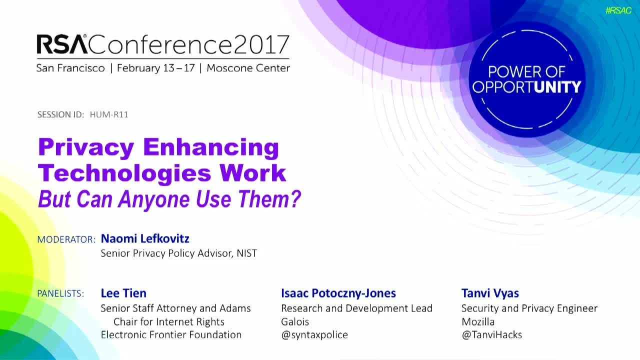 Let's Encrypt is basically a CA that we do with Mozilla and several other partners, and the idea is to enable webmasters and websites to more easily get certificates so that they can do HTTPS. And you know, we've got a lot of certificates out there now and part of what we were trying 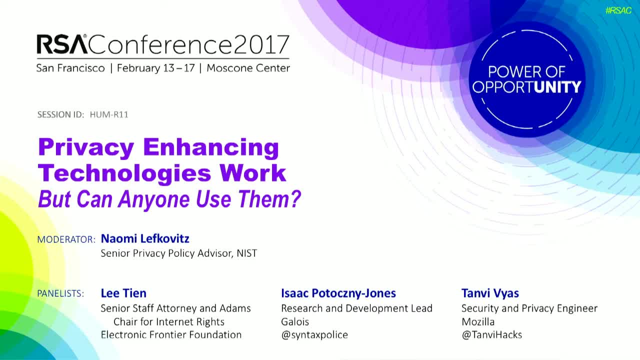 to do was to make sure that it wasn't just the big sites that everyone goes to that are technically very, very competent, but rather small sites that you know might not even really have understood what HTTPS is, and to enhance their ability to provide users. 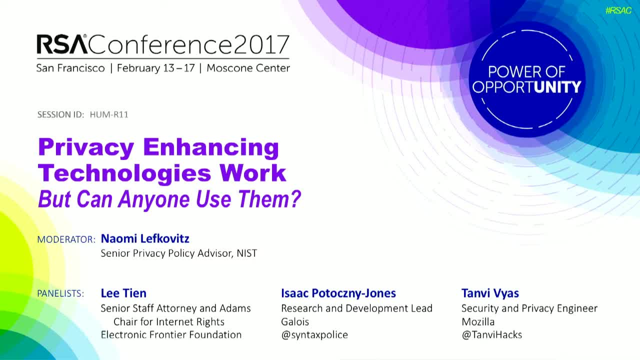 with at least a little bit of information. So you know, we're trying to make sure that we're able to provide users with at least that level of encryption between the client and the server. So all of those things in my mind are forms of privacy-enhancing technology. 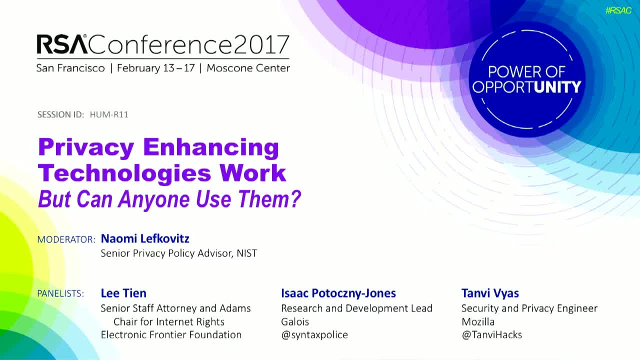 I can say: actually, my development team uses Let's Encrypt every day and it's changing the way we interact with HTTPS on the internet, because we can dynamically generate certificates for new services as we stand them up and turn them off, And it really works for programmers. 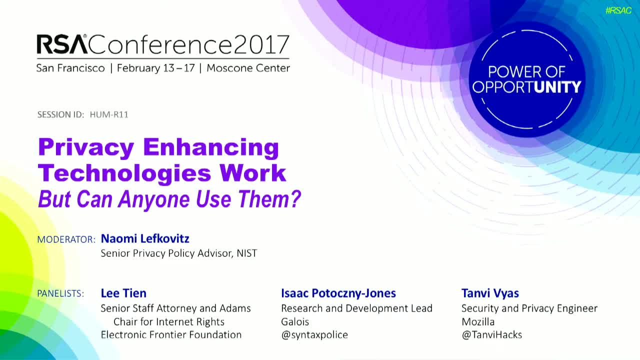 And it's a great example of what I was saying about really building privacy-enhancing tools for programmers. So I think that's a great sort of segue into my next question, which is: you know, I think sometimes people think about a privacy-enhancing technology like something like you know. 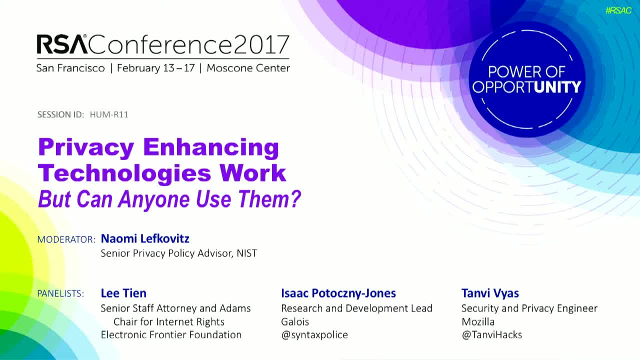 Tor or something where you have to go and users have to go and download something or set something up and sort of you know, stand alone or bolt it on, Right You know, versus something that's really baked into the design. I mean, is there a right way to do privacy-enhancing technologies? 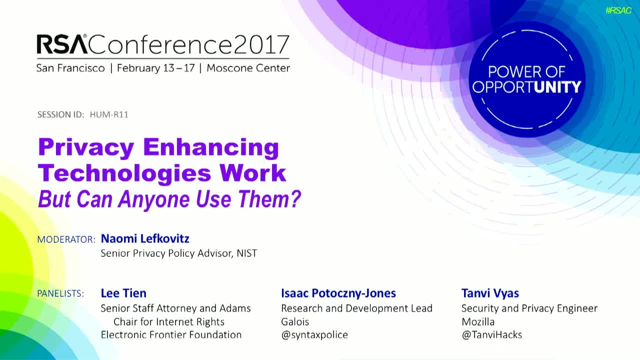 Is one better than the other. So, as Lee mentioned earlier, if Privacy Badger hadn't surfaced that there were 60 trackers on the page, he wouldn't have known. So, with standalone privacy-enhancing technologies, if the user isn't aware of them, if they don't, 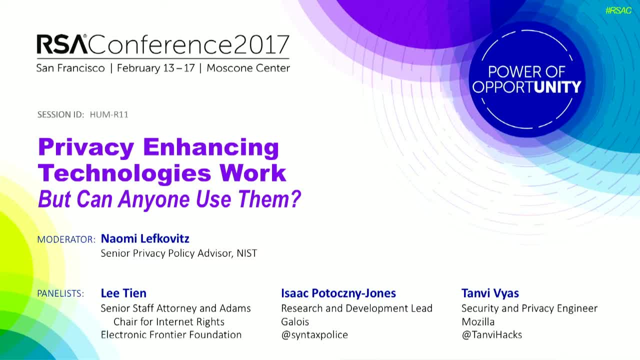 know about them, they're not going to install them, They're not going to use them And they're not going to benefit from them. But if we can integrate privacy by design into the software itself, then we make it available to more users and make it more impactful. 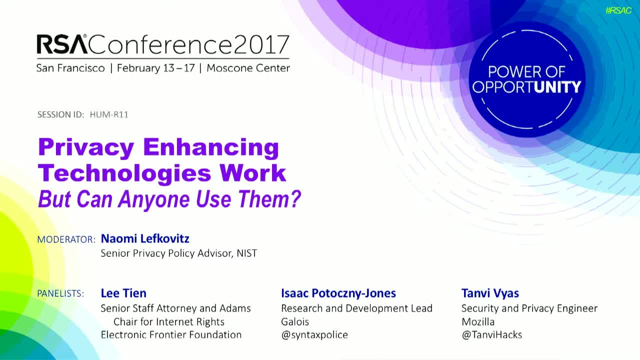 And we don't necessarily have to turn it on for all users. We could just let users know, hey, there's 60 trackers on this page, kind of as education, And then they could make that choice for themselves whether they want to block those or not. 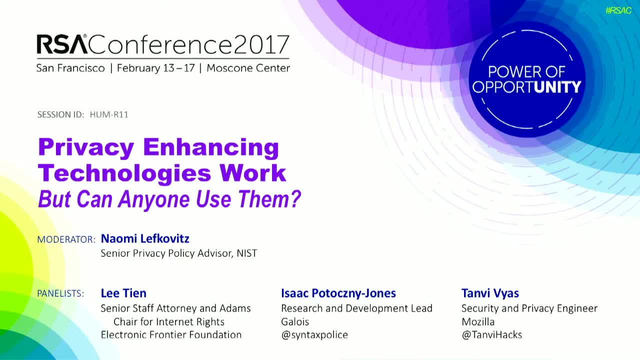 And I should make clear that you know, because Privacy Badger is an educational tool, it's not just a tool. Privacy Badger is a third-party product. Whether we're able to interoperate, to plug into a browser is you know, it's not up to. 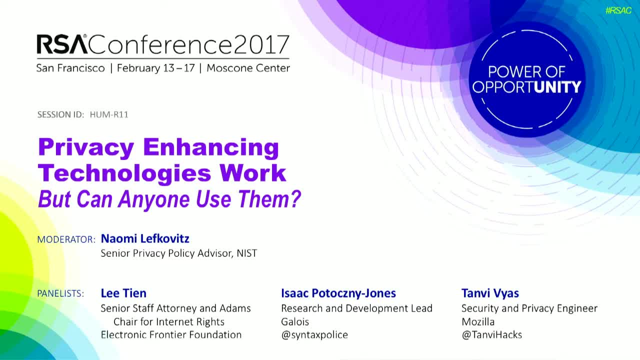 us. We write it, but we can't control that. If we can't get into a certain place to put something on an iPhone browser, you'll never get Privacy Badger on your iPhone browser. If you have an open-source browser, then that's going to be very different. 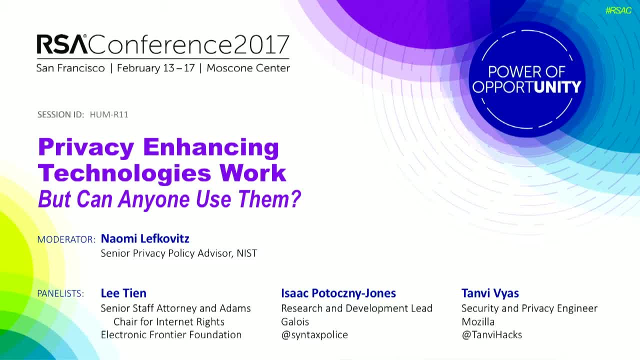 We'll be able to design and write for that And anyone will be able to get in. So there are all sorts of sort of important issues to consider when you're trying to think of how you get the right reach and what's the right form for your career in technology. 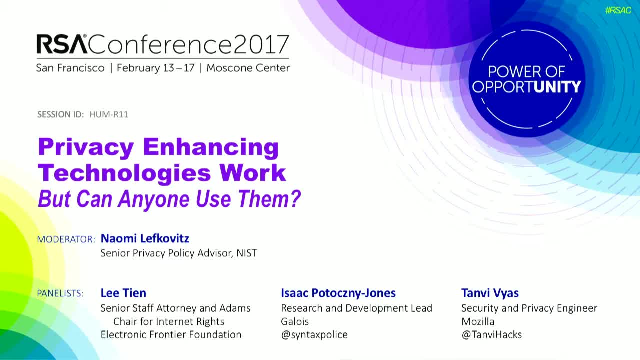 I think one of the challenges in privacy is that, similar to security, it's taken on this kind of adversarial model where it's kind of the users are desperately- or not so desperately- trying to protect their privacy, And I think that's a big challenge. 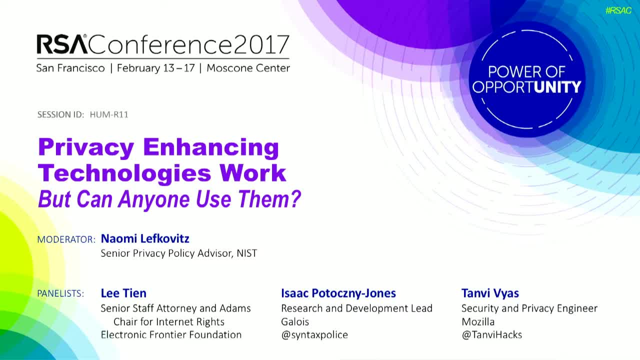 Yeah, And organizations are in many ways fighting against them. The user blocks cookies and then another organization starts to build these much more persistent cookies. It's kind of an arms race, and it's a losing arms race for the user because it's you. 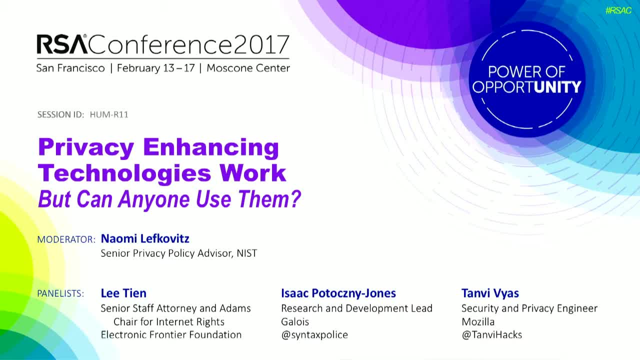 know it's the user against the people who are building the software that the user is using. So there's really nothing you can do. So these, you know, post-hoc tools are very important and they serve as a check against those problems. 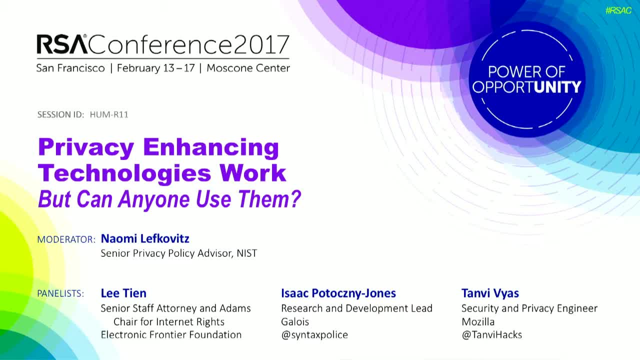 But I would definitely encourage anybody building software to think about building in security and privacy as a foundational technology. One of the examples I like to give of this is the whole concept of having a user account. So all of our computers, all the websites we go to, and even, you know, browsers are. 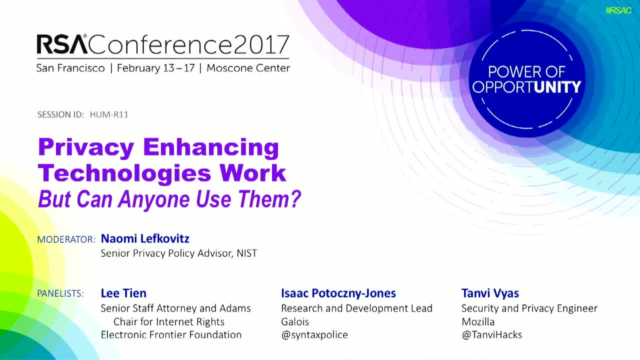 starting to have this concept of having a user account. It's even built in deeply into some operating systems And it's actually privacy-preserving technology. It separates my data from other users' data and there's probably some kind of security mechanism, like a password, to prevent other people from seeing my stuff. 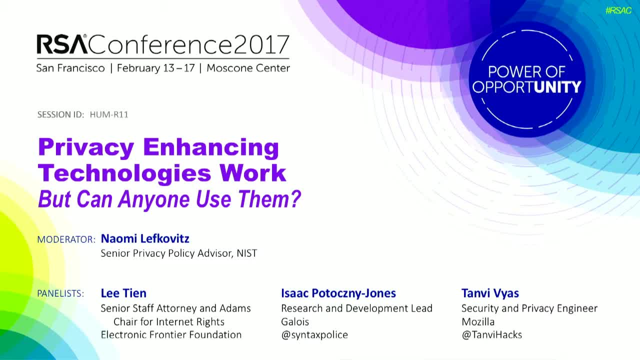 And nobody really necessarily sees this as an impediment to innovation or to financial success in your business. It's just something we build on top of to build better systems, And it's just a good abstraction. So I think we should work to find good abstractions like that that can benefit the users and not 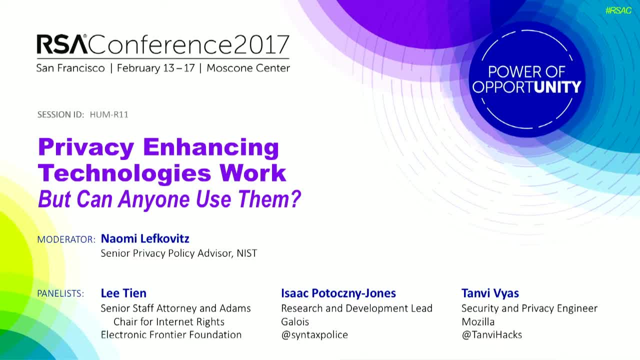 get in the way of our systems and build privacy in from the ground up in that way. And I'd also add, just on the issue of privacy design, we're obviously big fans of that, Yeah, But we know that it's not practical in all situations and one of the biggest problems: 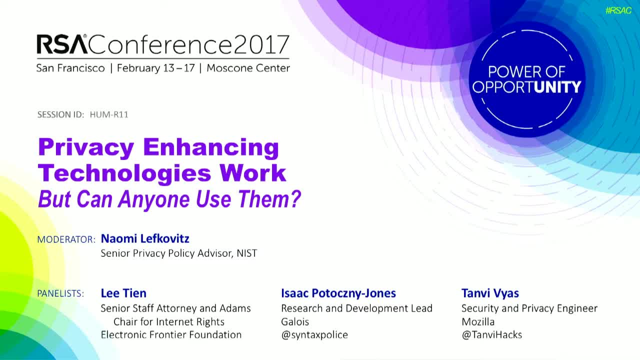 is going to be. you know a business model, right? I mean, if your business model involves trying to collect a lot of information, well, you're not going to design a whole lot of collection limitation into it, Or you know your privacy or policy. people might tell you that would be a great idea. 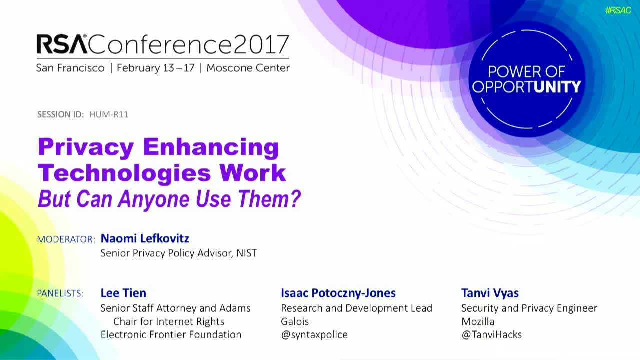 but your business folks are not. So you know this is, This is a long, you know, standing problem. The other problem is the convenience right. I mean the example I always use is back in the day, you know, when I had an answering. 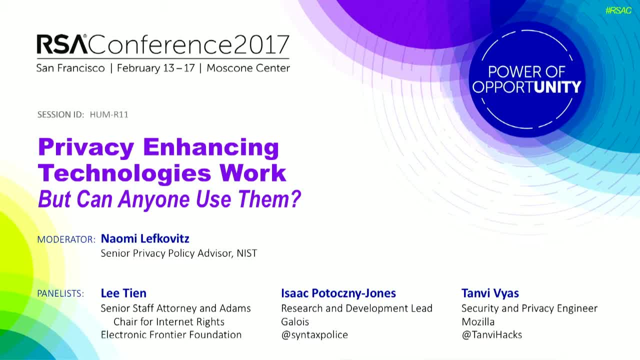 machine. it was a monomicrocoset and it was in my house And by design- And not by design just by happenstance, because the telephone system didn't offer me its voicemail- This was the only way to go, but it happened to be pretty private. 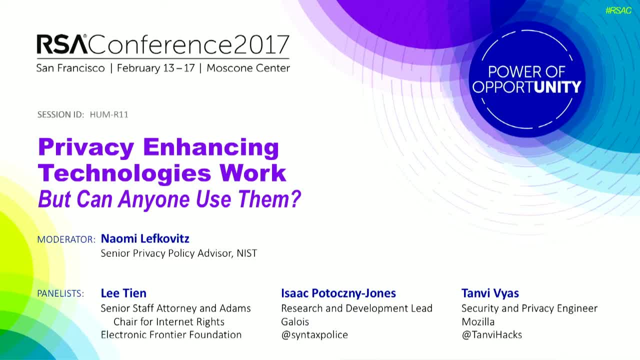 Whereas now all my- Yeah, All my- voicemail is sitting at. you know my carrier, I cannot control it. They can share it with anyone without my knowledge. It's convenient as hell because it's easy to get from anywhere, but you know that. 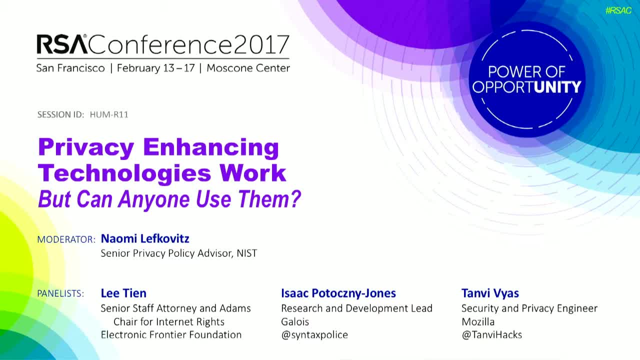 simple sort of change really completely alters the contingencies of information control, which means it affects my privacy. Okay, Thank you, Thank you. So let me follow up on something you were just saying, Lee, about, And I think it sort of goes to what you were saying Isaac. well, it's this sort of adversarial. 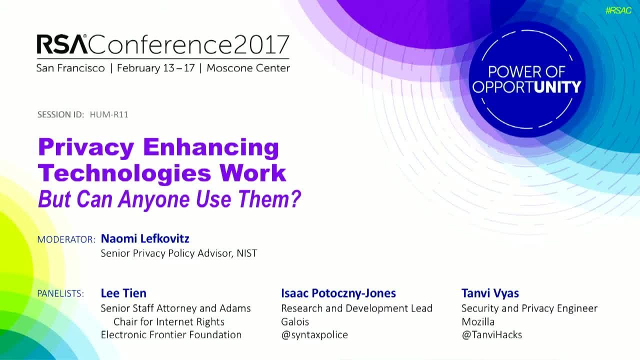 relationship around privacy, And I mean, you know I could see this as a definite challenge, but is it also potentially sort of you know, a lack of awareness or a lack of you know good solutions or privacy-enhancing technologies right? 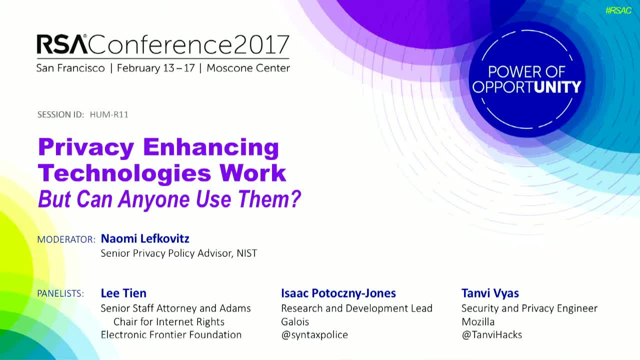 I mean you say organizations might want to collect a lot of information as their business model, but perhaps the primary issue is that actually they want to, you know, derive value or benefit in some way, which they also presumably think helps benefit their customer. 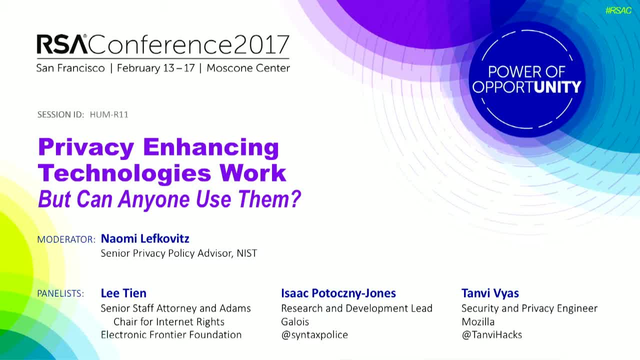 But what if they had ways to you know, derive value, access that information without actually having to collect it? right, I mean, you know, Yeah, I mean we can talk about cryptographic techniques. right, that could be privacy-enhancing. 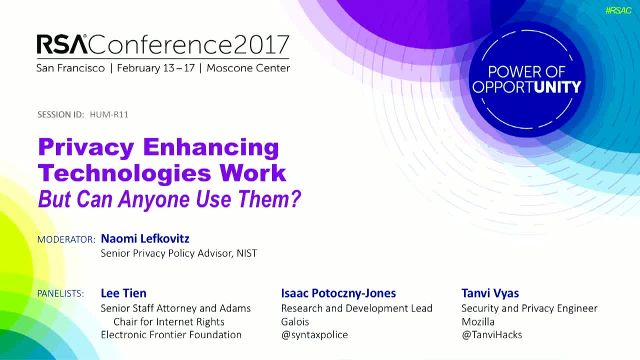 So I just, you know, sort of throw that out there to see what you think. Is it really the business model or is it the lack of, you know, awareness and good technologies out there that could actually help organizations do what they want to do but also protect? 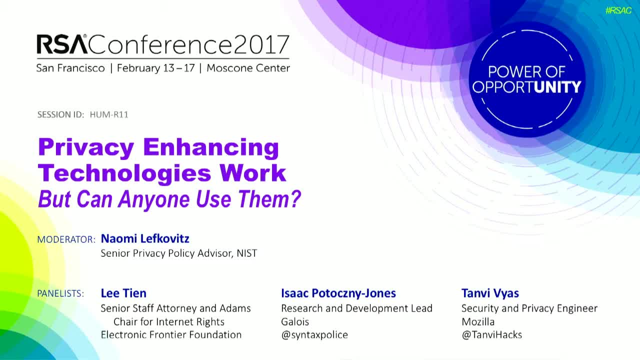 privacy. Isaac, you want to Sure? Yeah, I agree, And I do think it's a bit of both. It's certainly To build, You know, cryptographic technology to enhance privacy into a system, especially into the core of the system, at the early stage, when you don't even know whether it's going to. 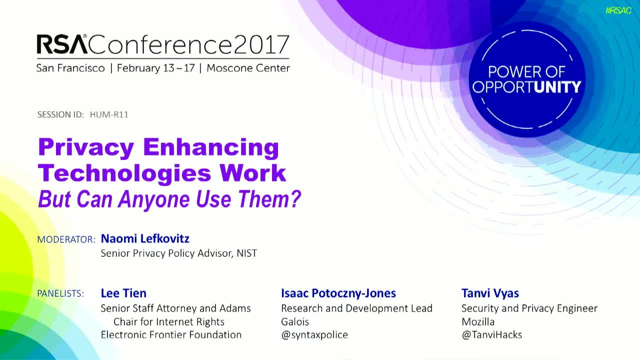 be financially successful and you're building a system based on functional requirements or feature sets that you really need and not focused on kind of you know, sideline things like privacy and security. So it can be really challenging in the course of developing products to do that and to make 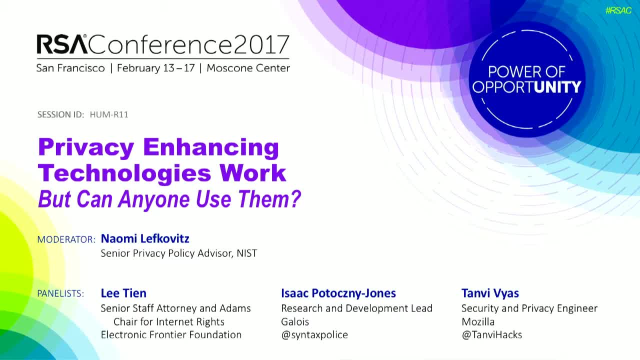 that investment in these technologies. But I think the first step is education, as you say, and I think NIST is doing a great job there- And I think that once people really choose to say, okay, we'll build these technologies into our systems. now what? 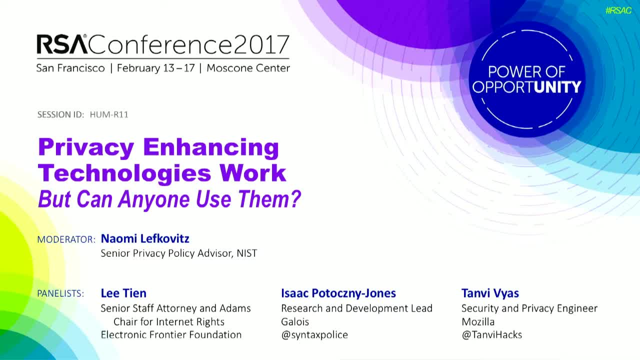 Right Now. where do I go to learn about how to do that? And I do think that's a real challenge. I don't think the information is all that readily available about how to think through these things, And I'll point to NIST's work at the NIST. 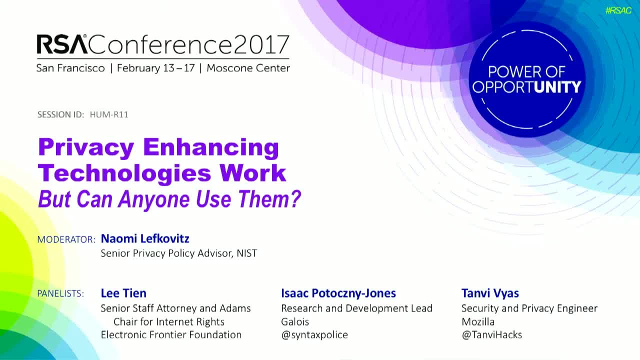 Yeah, Yeah Yeah. The privacy risk management framework is being a great example of new work in that area and you worked on that and I think Sean, who I think is in here somewhere, also worked on that, So definitely that's really important work. 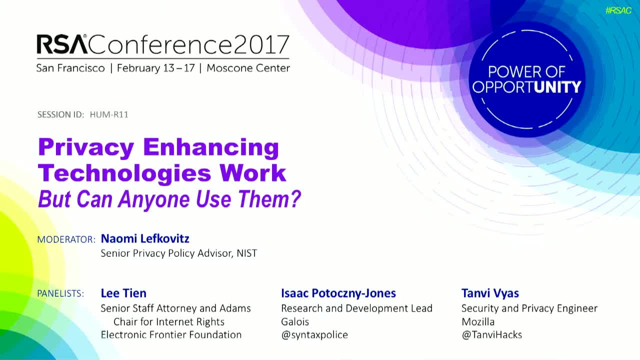 There's no incentive, right? There's no incentive for industries to collect less data or collect data in a privacy-preserving way, And so why would they spend the effort and find the right crypto to do that? Not only that, I mean because of just the. 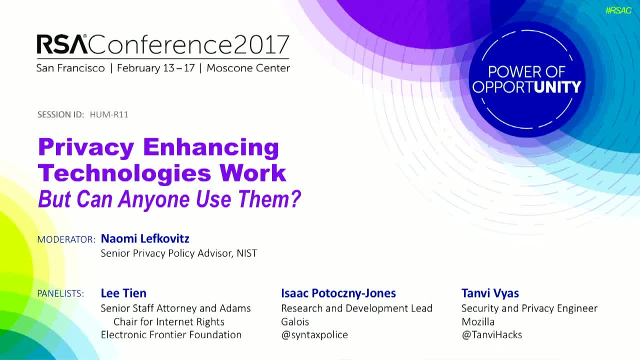 Yeah, There's sort of a temporal asymmetry because you start out, it's new, you're collecting data. Once the industry matures, they may mature around or begin to standardize around, something that's fairly promiscuous in terms of data collection. 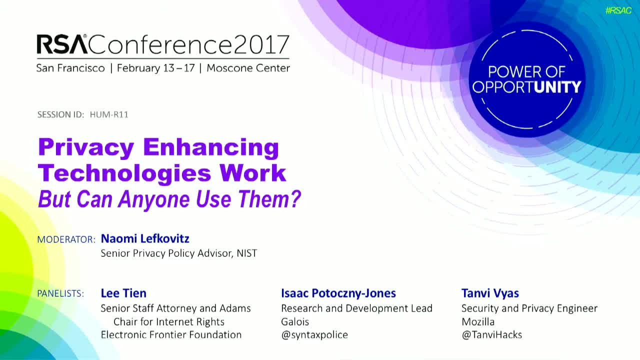 And then you run in. then you might in the next phase say, oh, that's problematic, But now how are we supposed to move off of something that's really just sort of a strong, stable equilibrium? right, It's a terrible equilibrium from a privacy and security perspective, but it's a strong one in the sense that if an industry member wanted to improve things, 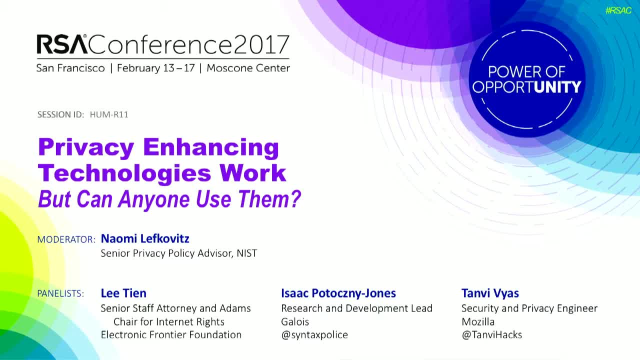 they can't pull away from the standard and they'll be spending money unilaterally to make themselves better when no one else is doing it. And the compounded thing which I really wanted to add in is that it really depends on the privacy threat in the first place, right? 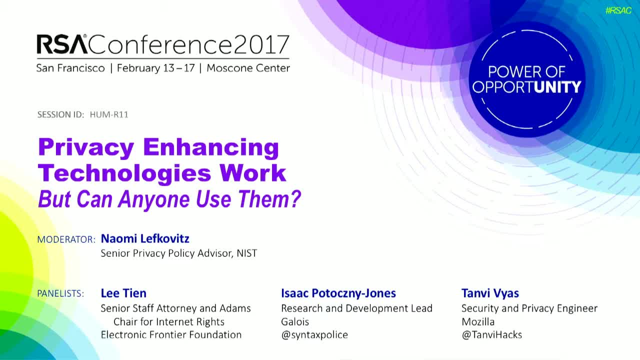 There are a lot of privacy threats that people don't know anything about, And so you might be the most fair-minded company in the world, but at the end of the day it's like man. they won't even see that I'm doing anything good for them. 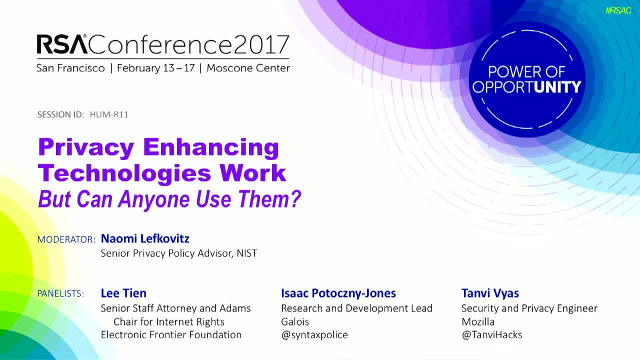 I mean, for years people did not understand or wasn't widely known that the use of cell phones was something that revealed location. You know over and over again court cases. you know we had to show this to people, that yeah. 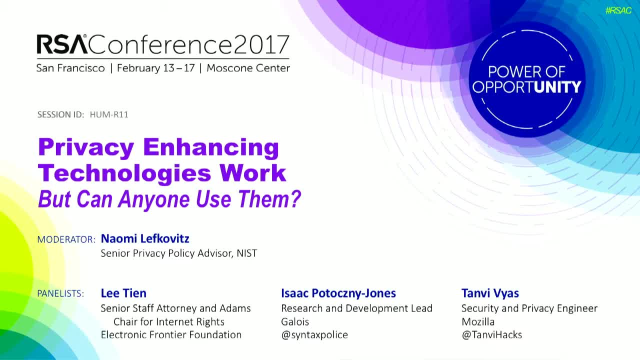 there's a lot of location going on, and then we had to sort of you know, argue about whether people knew it or not, And eventually the court sort of gathered that yeah, people don't really understand that, And so you know now we can treat that as protected. 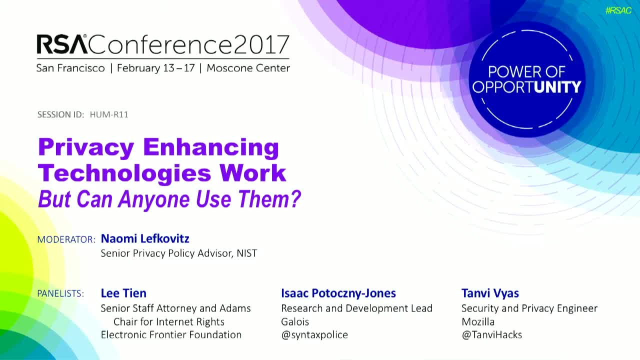 But you know, we understand when our laptop, we use our laptop, our cameras. we understand light and seeing. We can understand microphones and listening. Do we understand the power of traffic analysis, the power of lots and lots of transactions? 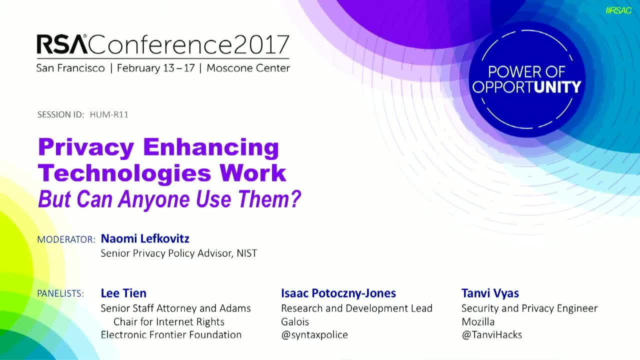 I mean, even today I go to campuses and I will talk about how you know the target pregnancy assessment tests and how you can actually get some pretty good inferences about whether a woman's in her second trimester, based on purchases at Target. 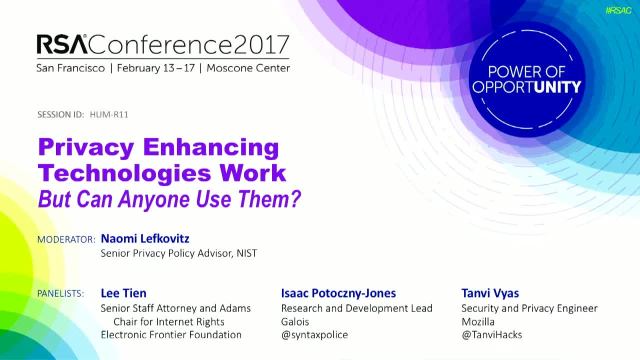 And you know, once you unpack it, people go: oh yeah, those things, they're all clues. But when you first explain to them they had no clue. They had no clue that this is a threat. And so if they don't understand it's a threat, what is a company supposed to? you know what incentive do they have to do anything about it? 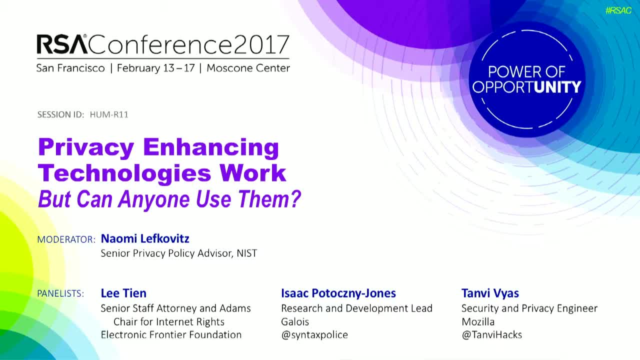 So a whole lot of the problem is also on our simple lack of understanding and awareness of how much privacy can be threatened by seemingly innocuous data. And people don't even believe or understand how much data is floating around in the economy, right, I mean there was a study done, a number. 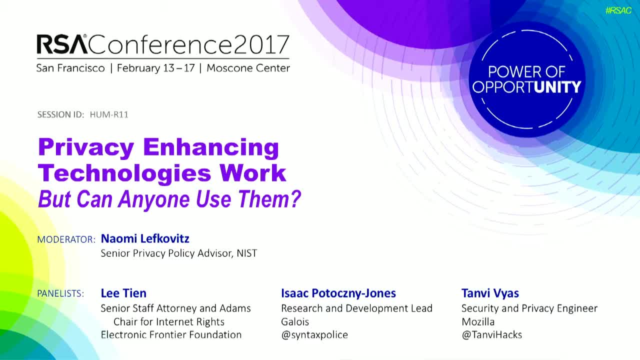 A number of years ago here in California relating to what people thought a privacy policy on a website meant, And it was a solid majority believed that if a website had a privacy policy- I think this might have been five years ago- then it didn't share information. 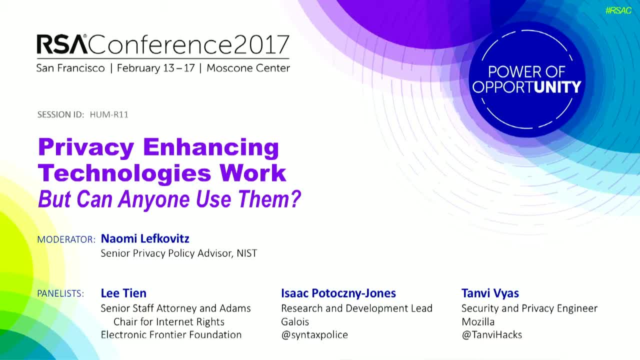 We all know that that is not the true case. It's never been the case. I don't even understand how people Could have thought that, But people systematically underestimate the privacy threat in the environment. And now we have the IOT and we have devices that don't belong to us but are you know, are in your built environment that are going to be collecting information. 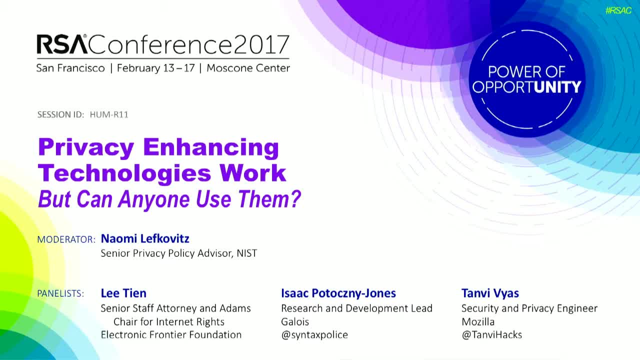 And you know, unless I can, you know come up with a way to you know sort of defeat surveillance In the, in the general public. I don't think there is a privacy enhancing technology that I as a user can use, and then I'm completely going to have to depend on the possibility of privacy being designed in. 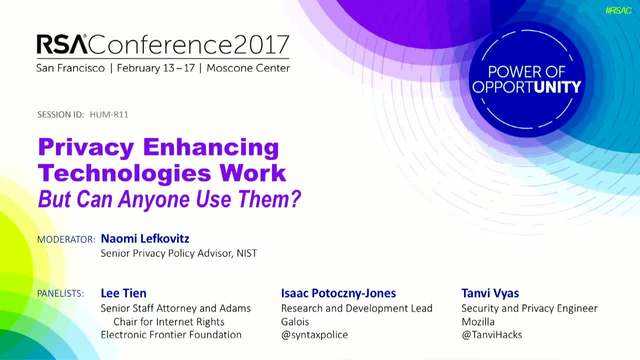 I think this brings up an interesting set of threats that are around, kind of statistical privacy attacks, where it's really hard for anyone to understand how much- as you say- how much information is out there and what you can do when you combine it. You provided that target example and 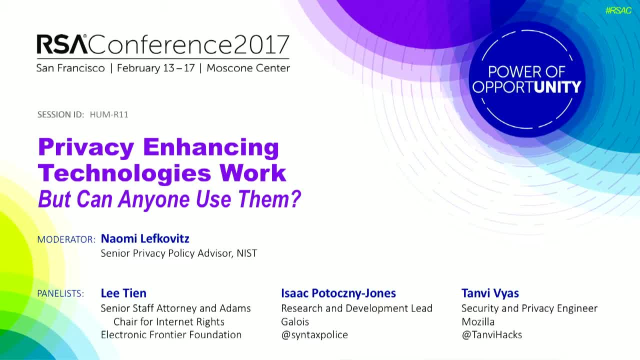 And another really fascinating one was where I believe it was. New York released a bunch of taxi data and I think it was just where you got picked up, where you got dropped off and how much the fare was and how much the tip was. And someone took just Googled for photographs of celebrities getting into cabs in New York City and they could recognize the street corners. so they could actually now identify based on just a photograph of somebody getting into a cab, find that ride and know where the person went, which was probably their home or something like that. 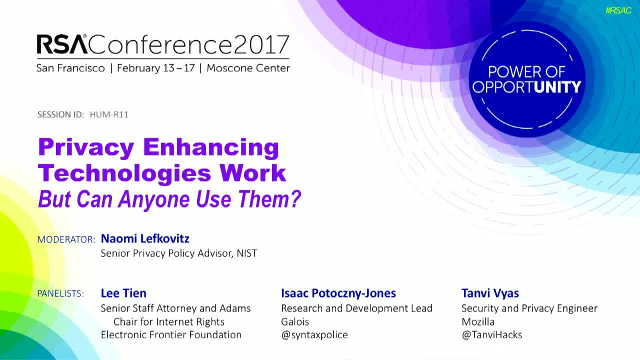 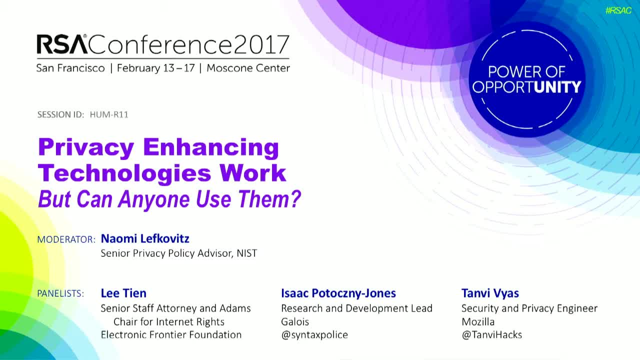 But when combined they are, they were completely show everything about the user's privacy. So it was. these things are really really hard to understand And, in fact, practically completely unpredictable, because you can have an unlimited number of data sets with this kind of information. 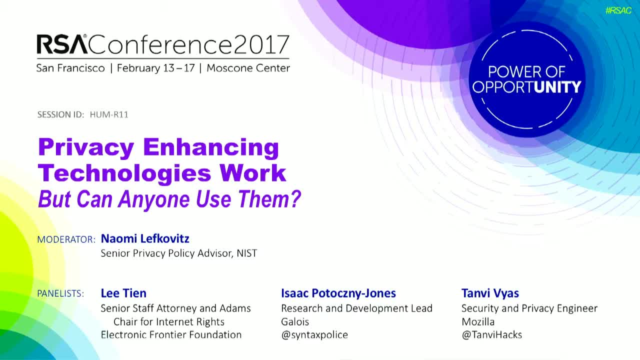 And so, especially in this kind of big data world we're going into, where IoT is a big part of that- it's going to be very hard to predict privacy threats. One of the other problems is even when users do understand that this data can be combined. 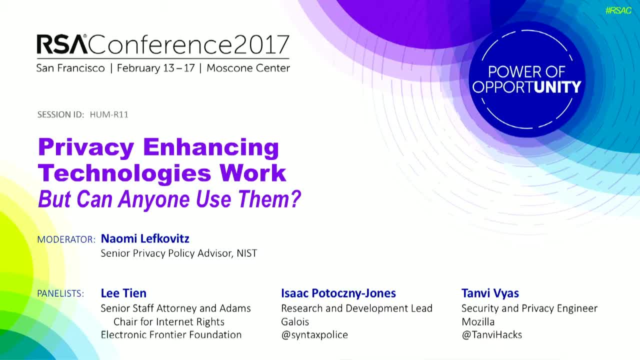 and you can learn a lot about a person from all this data that's out there. they don't understand what the consequences are. They know it makes them feel uncomfortable. They don't like that. this data is out there, But if they don't feel like they're doing anything particularly wrong, 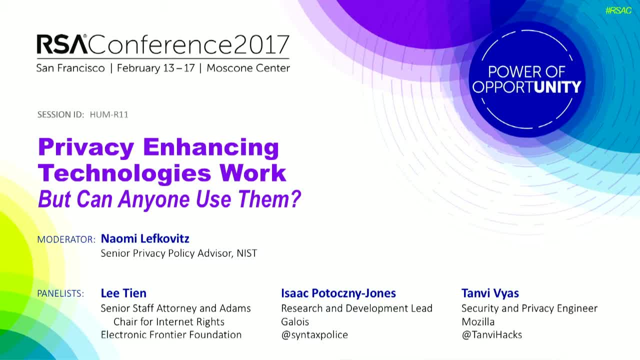 they don't know what the consequence to themselves will be, because this data is out there. So sort of following up. then you know- and I think you sort of framed it as you know, some of these standalone technologies that users can add on or download act as a kind of a check right. 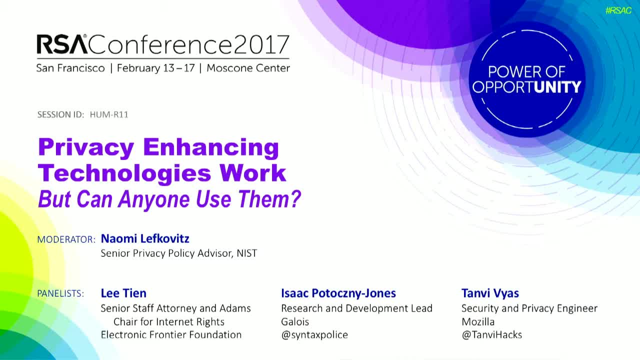 in some of these challenges. You know what about some of the challenges, What about some of the lessons learned in you know, users' ability to, you know, actually make these technologies work. I mean I think Tor is commonly cited, as you know, kind of intimidating right for the average user. 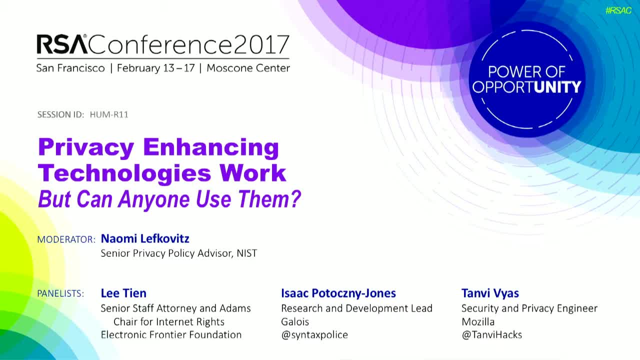 So you know if you want to speak to that and some of you know your work and some of your lessons learned in trying to implement these. Yeah, I find that often we design for privacy. So we have Tor, which is very private, has anti-fingerprinting features, blocks cookies. 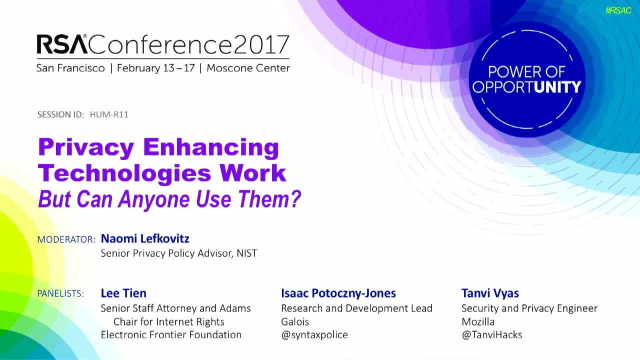 uses an anonymized network, or you have a standard browser that doesn't have any of these things, And in the standard browser you try to put as many privacy-preserving features that you can by default. but as soon as anything breaks an experience or a page, you stop and you say, well, we can't have that. 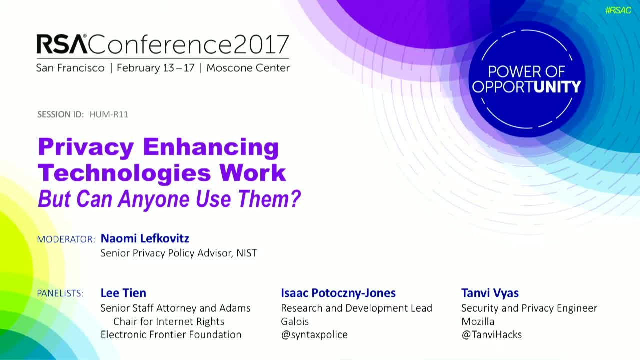 We can't have broken pages. So you There's these two extremes of either a completely locked-down mode or a completely open mode, And I think what we need to do is bridge the gap there and have more of a dynamic mode, a mode where a user can opt into additional features and control their privacy. 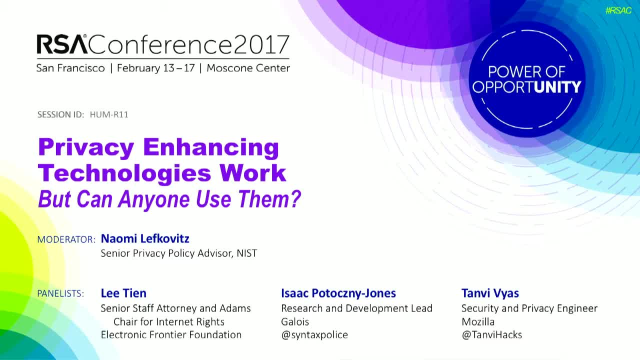 And, in cases where they do experience breakage, have ways for them to recover, have ways for them to say: okay, I'll turn off privacy for this site or for this or for this hour, for the moment, so that I can use the full feature set of this web page. 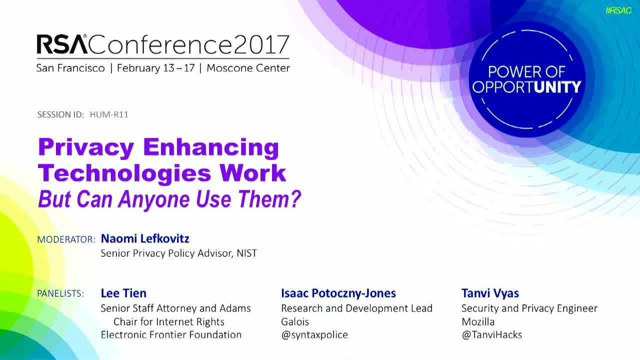 And at that point they're making that choice, So allowing the user to make the choice between usability and privacy instead of this all-or-nothing, all-the-time kind of situation. And so the Brave browser has this idea of shields up, where you turn on a bunch of different features that increase your privacy. 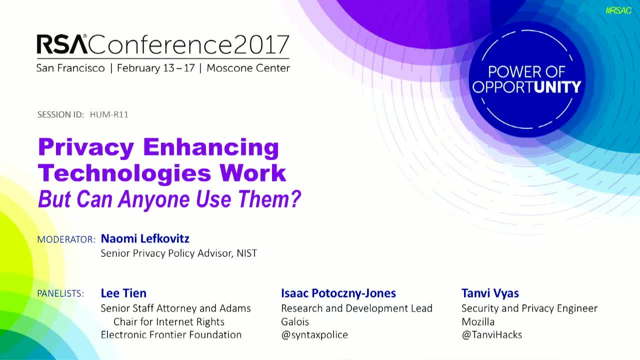 and then you can put shields down on a particular site. So that's an example, And I also think that technologies are not designed for users that have the appetite for this poor user experience. right, There is a class of users that are okay with the poor user experience in favor of privacy. 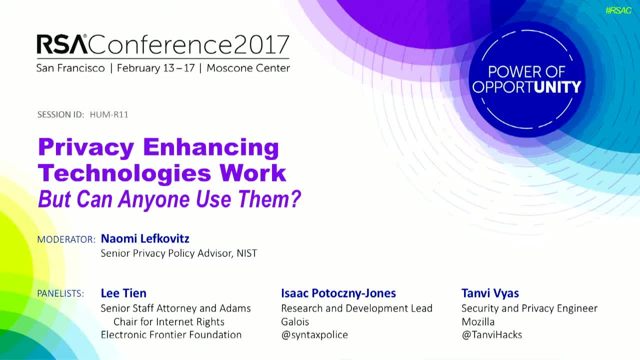 as long as they can recover from it, And we find that technologies are designed in these extremes. Either you have Tor or you have a regular browser. Yeah, I really like. I think that's really accurate And I think that it's very difficult for any of us on a day-to-day basis. 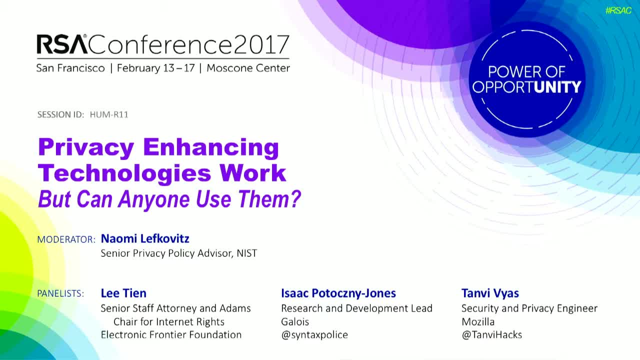 to really operate in a private mode, in a private way, throughout the digital world, because we want to use our browser features that remember our browsing history. We want to use cookies so that we don't have to log in every time we visit a page. 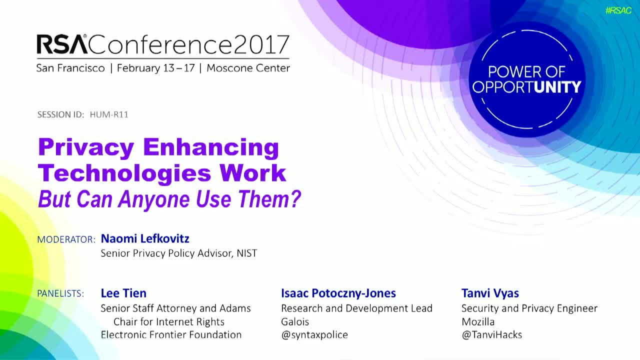 And our phones. you know nobody is going to really practically be able to lock down their digital life so that your privacy is not getting violated. The only real solution is not to use, you know, a smartphone, And I don't think that's acceptable to most of us. 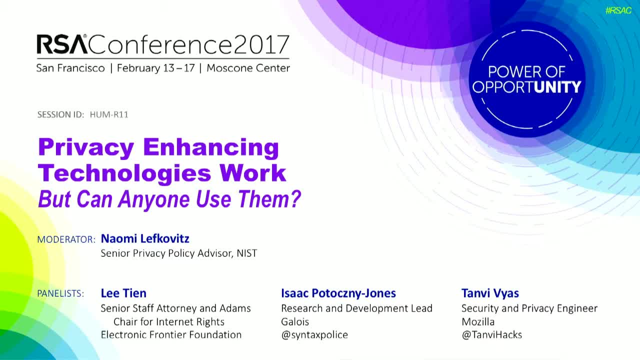 And so I love the kind of features, like Firefox has, of the kind of private browsing mode where you can switch into that, And I think that the you know lesson is to you know how do we apply that to, whether it's personas or something else? 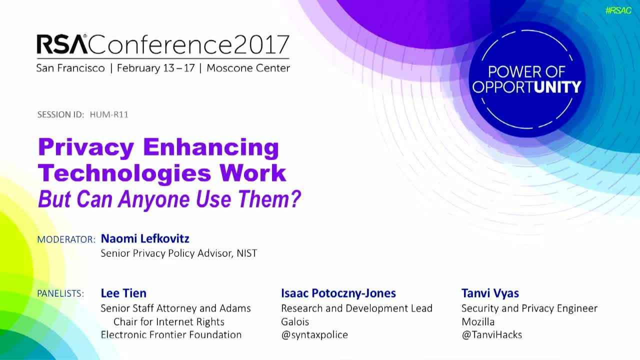 but choosing areas of our lives where we're you know we're not going to be able to do that. We choose to be private, And maybe it's not possible to be private 24-7, but to say there are these separations I want to make between my business life and my personal life. 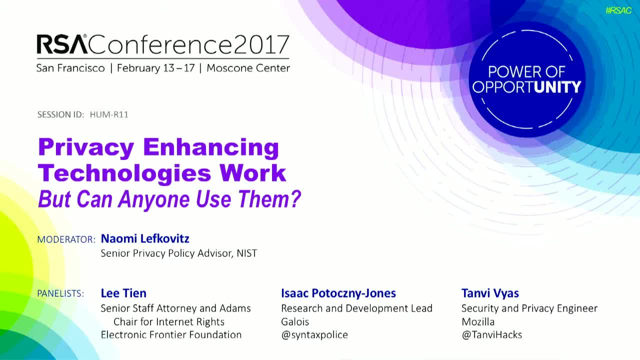 or my health care or my love life or whatever it might be, where you are, you know, particularly choosing to go into a mode that shields up or that's privacy preserving and maybe encouraging users to think more along those lines, while at the same time trying to get the industry to move in a way that's more preserving user privacy. 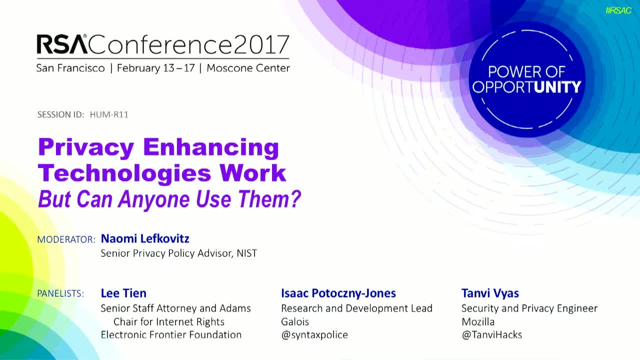 But I think, switching to this way of thinking and saying, I'm going to use a different- you know- user on my computer, a different persona on my phone, a different mode in the browser or, to the extreme, a completely different set of even hardware. 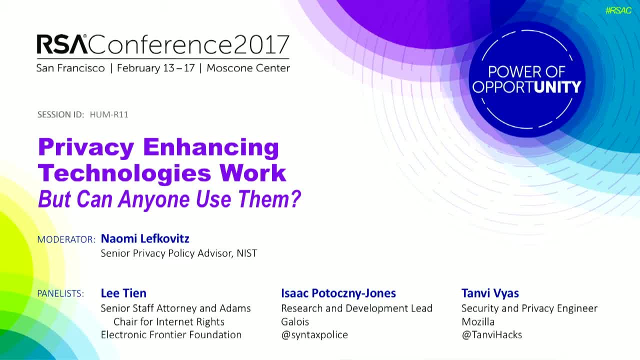 I use a different laptop when I go to some security conferences, for instance. So we have to probably shift to that type of thinking. I think, And I think that you know, this is also a reason why the privacy enhancing technology by itself is always going to fall short and it needs to be combined with, you know. 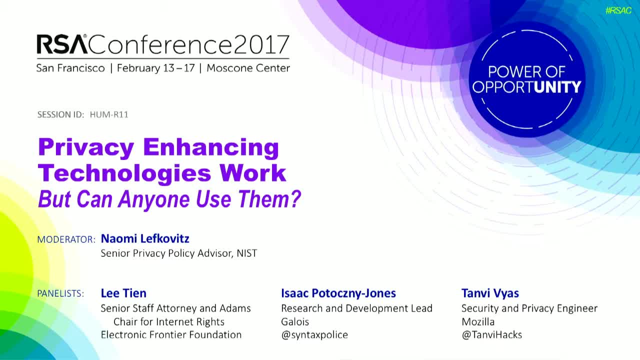 just like in any sort of security concept, you want defense in depth. you are not going to rely on any one particular component to do all the work. The privacy enhancing technologies can be useful for certain kinds of surface disclosures and certainly useful for collection. 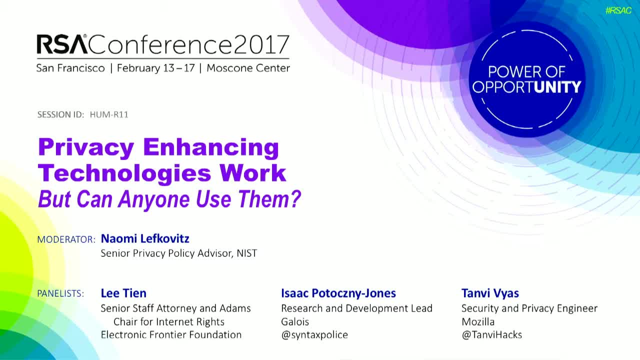 But you know, for instance, one of our products is Privacy Badger, and it has this. It has this ability, as I've described, to show you what's tracking you. It has also the ability for you to decide, then, what you're going to do about it. 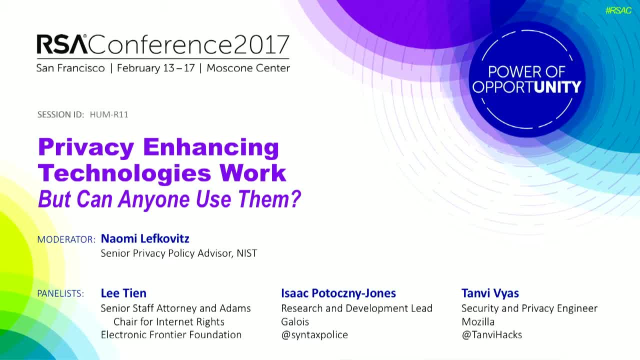 And we've paired the Privacy Badger technology with our own do not track policy, And so you know. the idea is that some use some websites, some hosts out there on the Internet are committing to through policies about collection, about how long they retain data, what kinds of 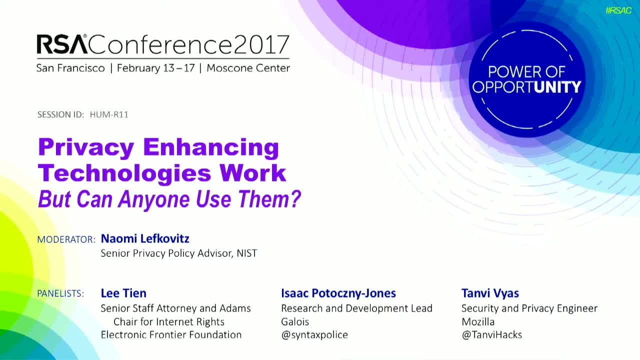 rules they're going to follow in terms of opting in requiring, opting in consent and sharing data, And these are, you know, these kinds of back end things, everything that happens after collection is very hard for me to imagine that a privacy enhancing technology, unless 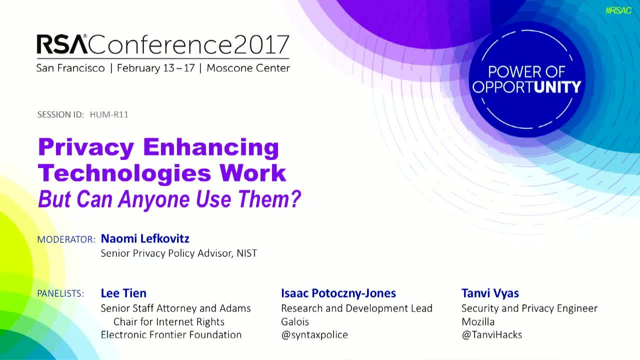 it actually, Yeah, is designed and meta-tagged, every bit of data that you sent and could somehow, you know, maintain, actually, pull it back. You can't control that Once you have made the decision to share that information with that website, with that host. 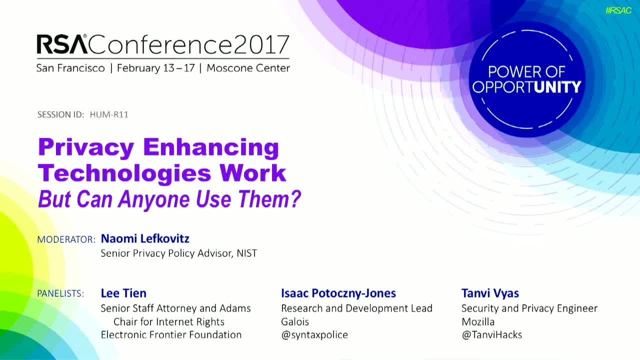 then they will have the ability to turn around and disseminate it elsewhere, So unless you can make it expire, But in any case, though, So there's a real role in all of this for the back end. Yeah, Yeah, So we have to understand policy kinds of rules, but there are the. 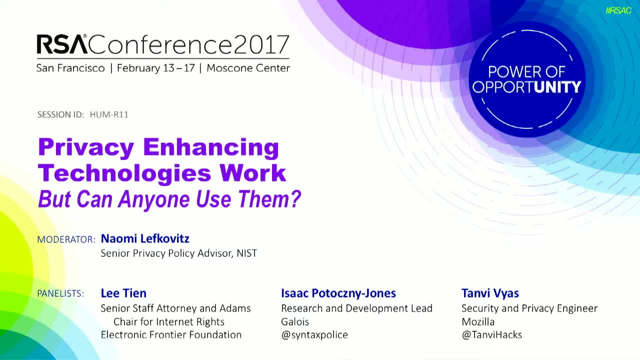 Also requires that companies, businesses and governments as well, you know- be transparent about what those rules are, to disclose things You know. if they You know, I would be much more inclined to share my information with an entity if I knew. 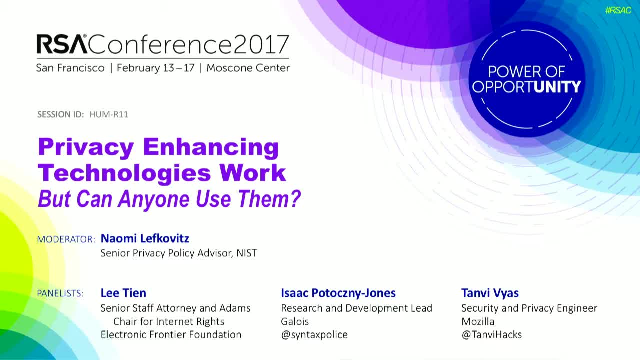 that they were not going to share it without my express permission personally, And that could lead to me, you know, engaging in a lot more transactions simply because I have a basis for trust, a verifiable basis for trust. Right now, we don't have a whole lot of that. 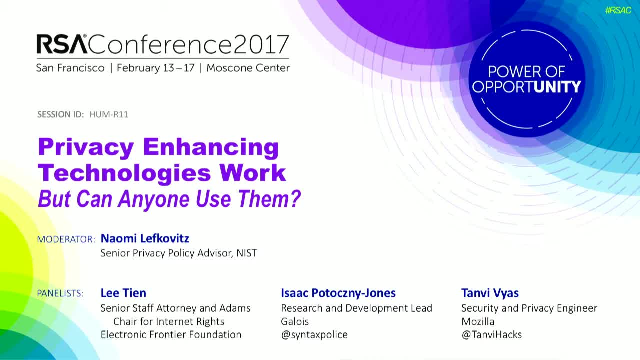 In fact, it's impossible to even know who's collecting the data for the ordinary person, So there's lots of reasons for them to not have any trust in the information system And, paradoxically, that makes it harder to have this in between. 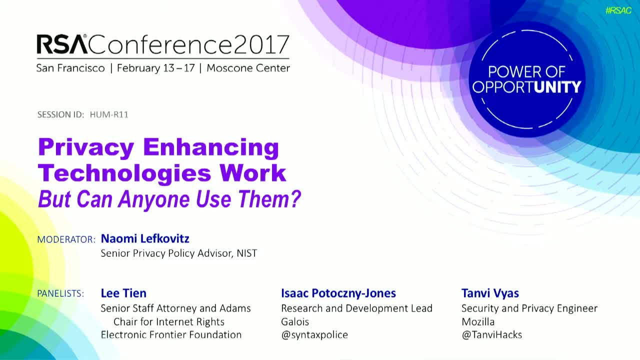 Yeah, Right, Because if it is the case that a single transaction with some website that is untrustworthy leads to, you know, all of your browser information and browser headers being captured and a whole lot of information gone, well then it is gone. 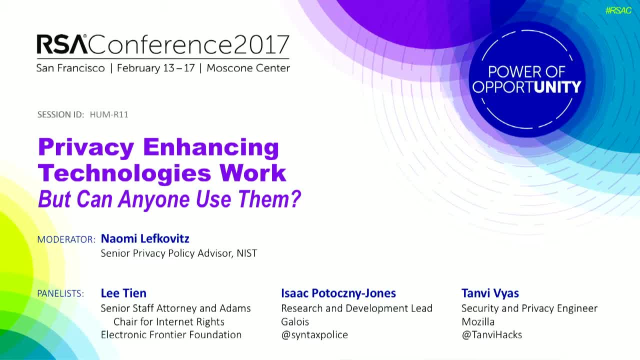 And in that case, in that sense, privacy can be like security, where it's only as strong as the weakest link, And so that makes it Tends to push the two ends of the The spectrum further apart rather than closer together. 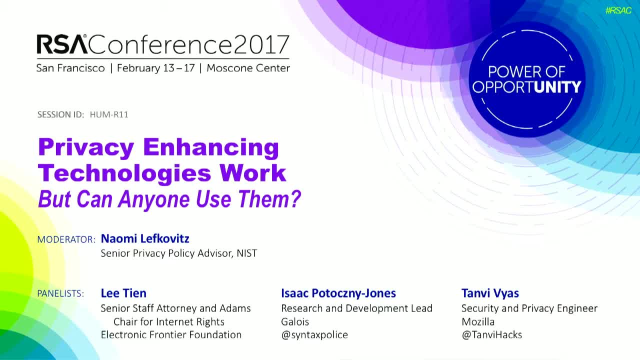 So I would submit that we need this complimentary level of legal or some kind of contractual protection in order to make the technological, Give the technological side enough juice. And people probably may know that in Europe they have the GDPR, which is a very strong 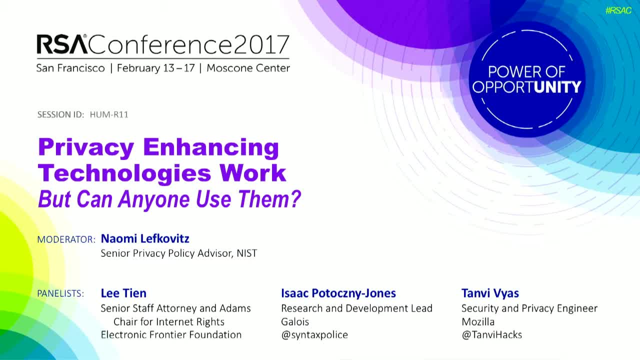 privacy rule about how data is managed. We don't have any type of rule like that here, Yeah, And I'm not sure we ever will. but I think part of the challenge with kind of the back end after collection and processing, how does that data get controlled? 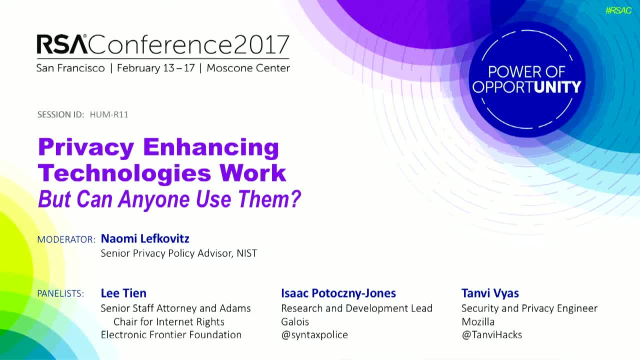 I think part of the problem really is that as a society we're a little bit suspicious of the idea of privacy. I think we You know, privacy and anonymity and security are conflated in these kind of odd ways. that makes us really not sure. you know the old, if you don't have anything to hide, what are? 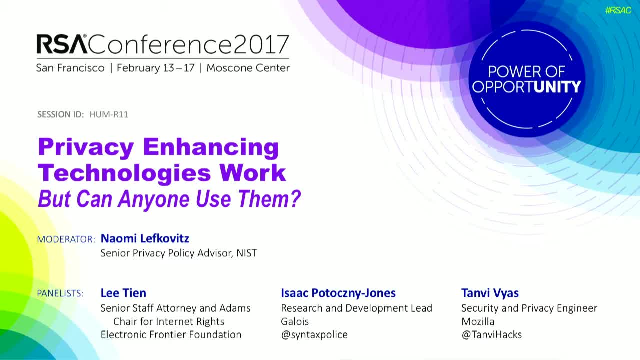 you doing right. So I think valuing privacy as a core American value is actually pretty important to making these changes, whether they end up being codified in contractor law or- you know just well- expressed in documents like what NIST put together about- you know, a privacy framework. 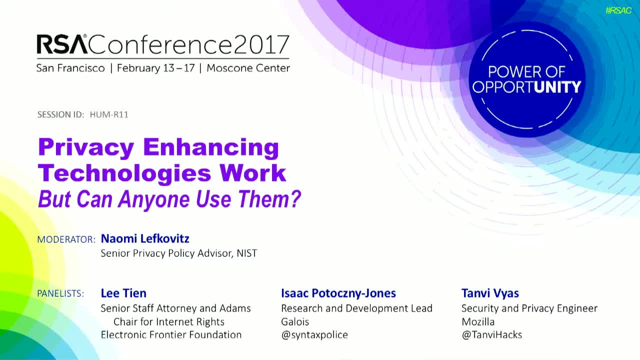 that says, at least, if you've decided to do a good job with privacy, you have a place to go to build it out. But I think first, as a society, we really need to learn to value it, And I think that's changing. 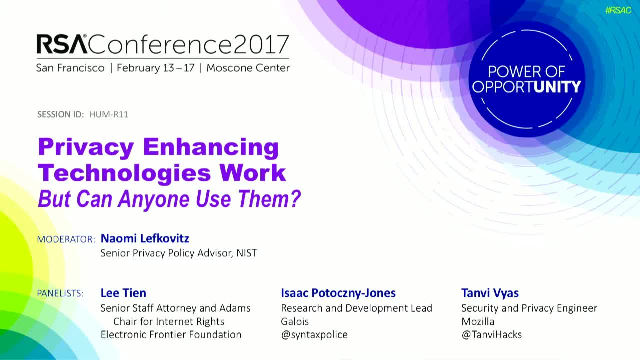 I think over time people are becoming more and more privacy conscious And right now it may be a small fraction, but as the world changes and things go on, in five years and ten years it might be a higher fraction of people And we have to be. 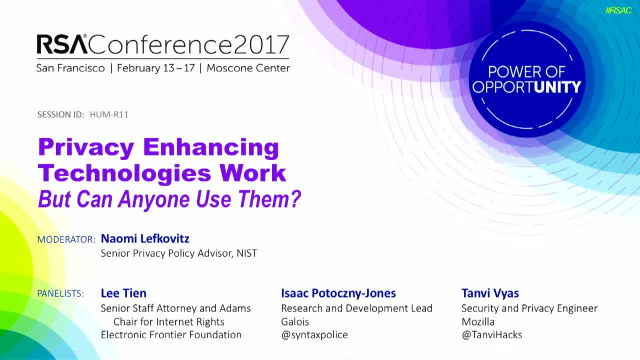 I think technologies have to be ready for that. So I want to make sure that people have time to ask questions. I don't know if anybody. If you can use a mic, that would be great. Thanks, Hi. I'm wondering: should users be skeptical or encouraged when we hear about companies? 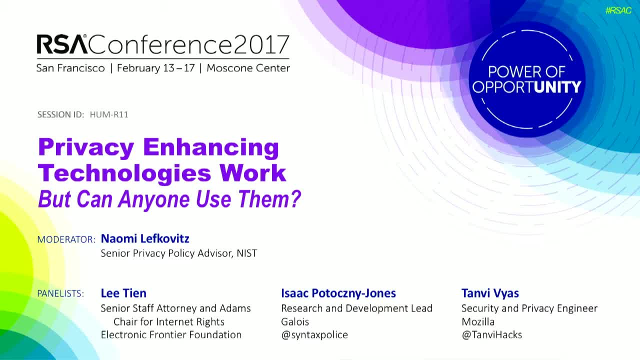 like Apple using differential privacy when they have all this data about us, Should users be skeptical of sort of big companies? I haven't heard about Apple doing work in differential privacy, but I believe you They have. They've definitely announced that they are trying to use differential privacy techniques. 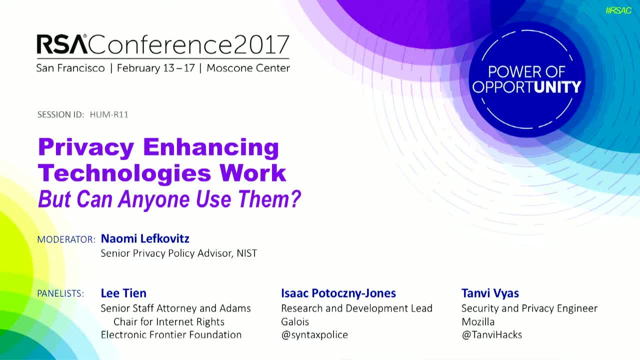 You know, Yeah, I've been encouraged and excited that they've stood up for privacy in many instances. But I think to your point about financial business models. you look at a company like Apple and what they sell and where they make money, versus a company like Google or Facebook. 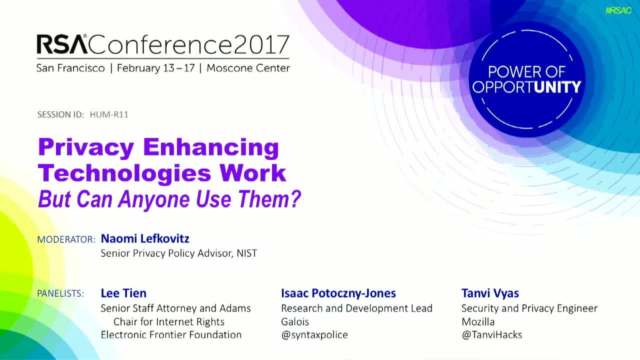 and what they sell and how they make money, And it's certainly a lot. I don't know what any of these companies are doing behind the scenes, really, but it's certainly a lot easier for Apple to sell laptop computers when And hold the line on privacy versus. 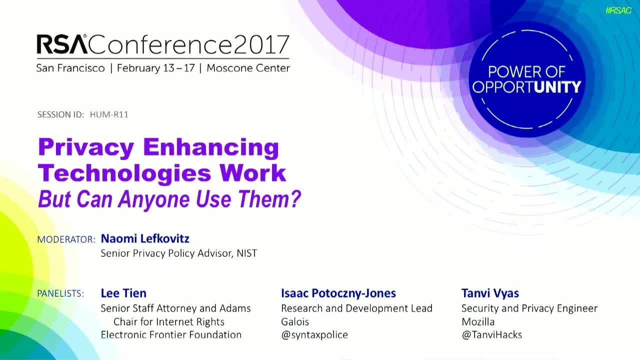 And hold the line on privacy versus organizations whose business model is collecting data. So I would take that into account. Yeah, Yeah, No, I mean that's This is. I always tell people be skeptical about the promises, but really the business model matters. 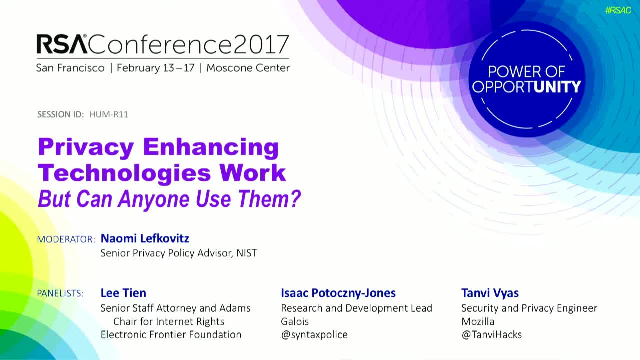 It's possible for companies to do things that go against their business model, but I would welcome if more did. But certainly what Isaac says is exactly right. Yeah, I mean, Apple is not fundamentally, is not very much of an ECS, of an electronic communication. 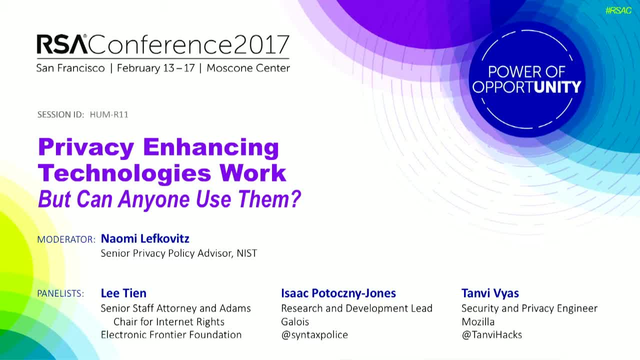 service. It is not very much of an ISP. It isn't someone that sits on a giant pot of user content and user communications that law enforcement is repeatedly interested in, the way that they're always going to Gmail or always going to Hotmail or always trying to. 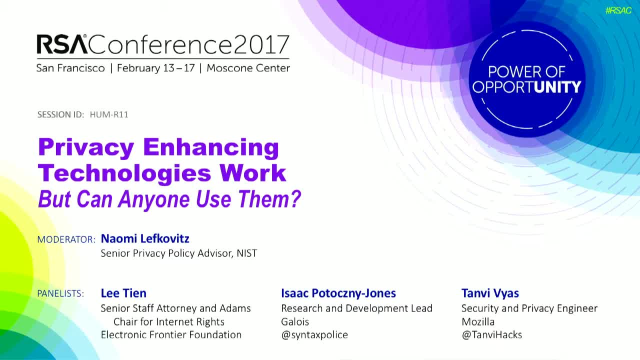 Trying to see what people are private messaging on Facebook. Apple isn't that kind of a company and similarly they're not as much an ad-based company. So again, the kinds of data collection they engage in and the importance of data promiscuity. 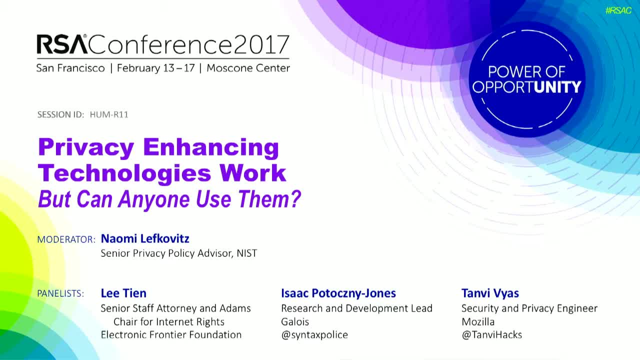 to their business model is very, very different, and I think we really see that with San Bernardino. They decided to make a stand, a public stand. Yeah, They decided to make a stand against the government on: We don't have back doors in our phones. 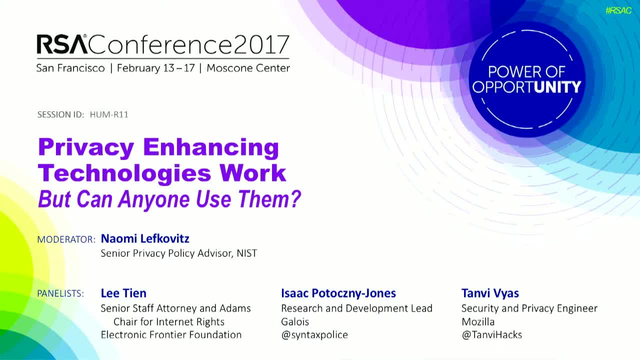 We are trying to keep that secure. The FBI was The government was savage to them on this for being it's just privacy PR and we don't really know what's inside, but it sure seems like they put up a big fight. that is technically. 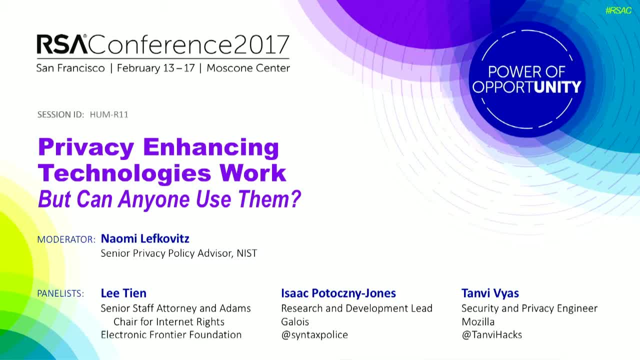 is challenging. They have devoted a great deal of engineering resources to them, So that's all very consistent. I mean. the reasons why they do it aside, it is good for the ecosystem. The Safari browser has more privacy-preserving features by default than any of the other. 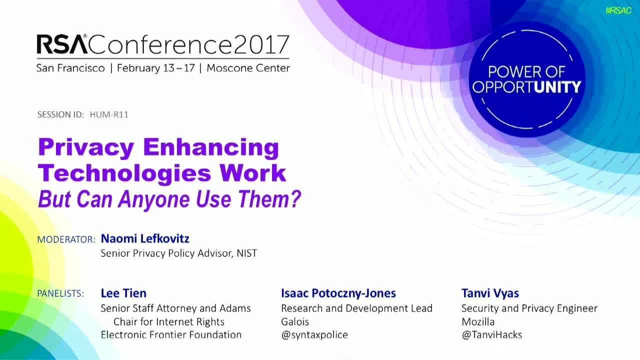 browsers have, and part of the reason for that is that Safari isn't a first-class citizen at Apple. That's not the way that they make money, and they get Safari by default on iPhones right, So they know users are gonna use that. 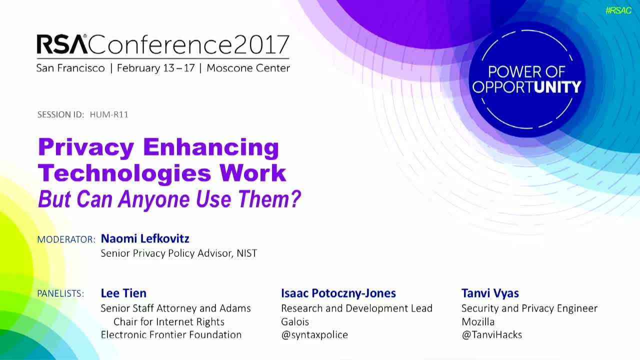 Yeah, Regardless. And that actually pushes the web forward, because mobile sites now have to tailor their sites to meet the privacy-preserving features that Safari has, otherwise they're gonna have users with broken experiences. Any thoughts on a strategy to get to improve our privacy consciousness in our culture? because 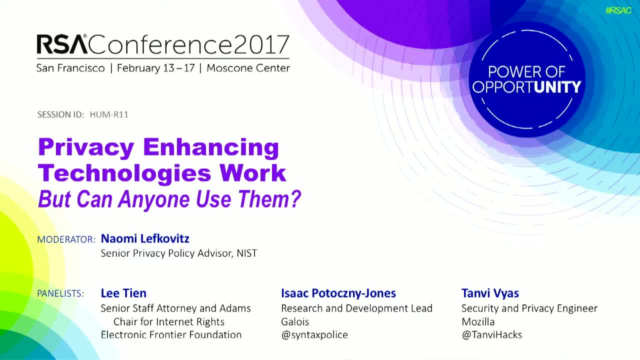 of you know哎S and absences of just giving up some part of your privacy to be able to ask, suck, Google a question and get a response- What was the Oscar-winning movie of 1974?? And they're willing to give up some of their privacy to get that silly answer. 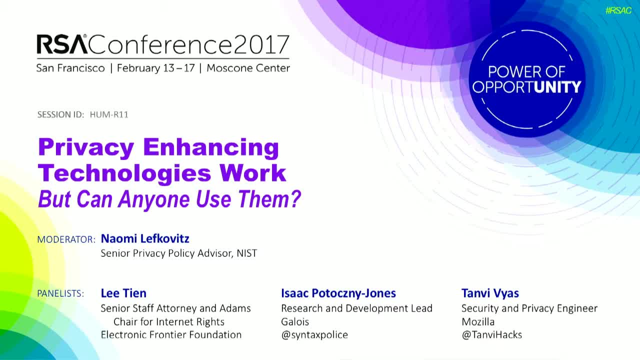 I think that's one of the issues that we have with the information age, as people don't want that information. they don't realize they're paying for it by sharing their personal information. Very fascinating, Yeah, Thanks. I think giving people better models is helpful. 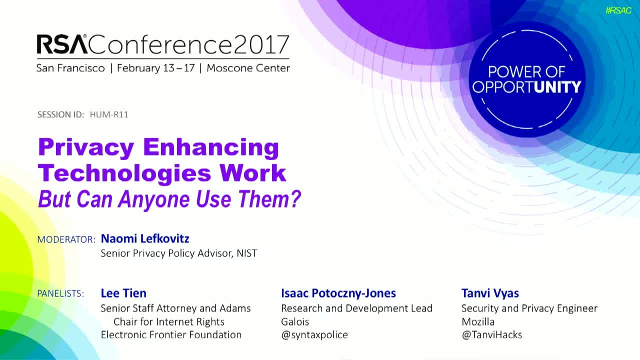 I like to give an example where, let's say, you're playing poker and everyone knows what your cards are, but you don't know what anybody else's cards are. That's kind of what it's like browsing the web today. I don't know that there are too many examples of this, but certain websites can vary their. 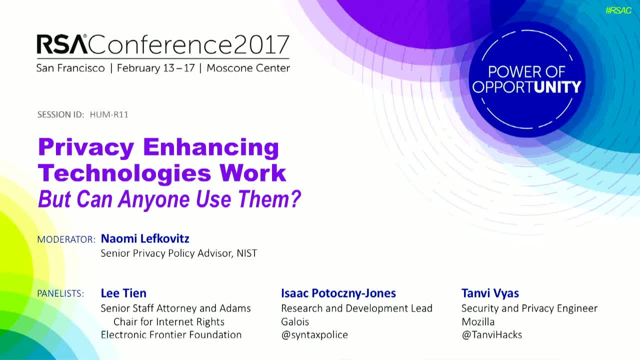 pricing based on what they know about your buying habits, And so people don't necessarily understand that information about them can actually be used against them in sort of a manipulative way, And I think that might be more motivating if people could really see and understand. 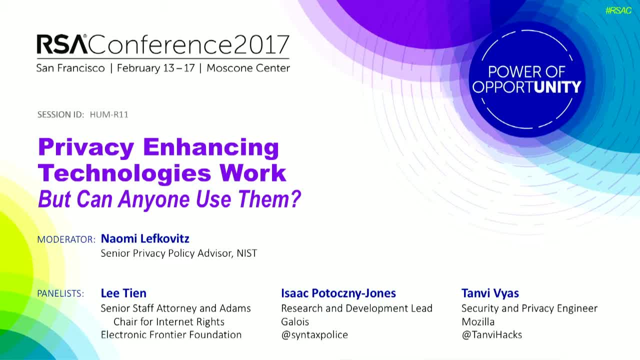 more examples of that, where people really aren't taking care of their best interests. But I think people need to understand that you can buy and sell personal information and then they have to ask them. I mean a lot of it. to me it's just really important. 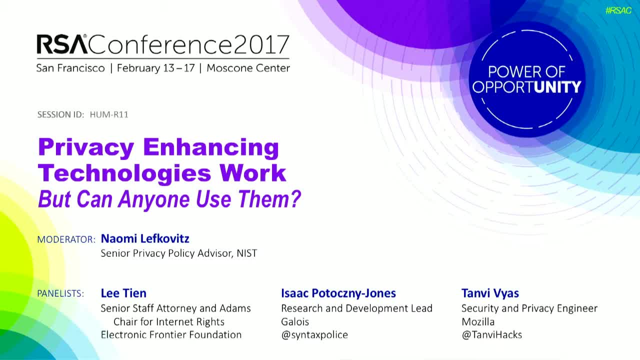 It's really sort of: what else would they do? You know? it's like, if you can imagine that you have, is there anything about your life that you would prefer that your employer doesn't know? If there is, then you can think: well, so is any trace of it revealable through my phone? 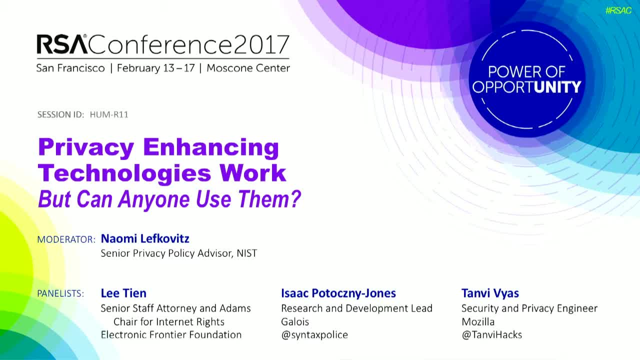 calls through my use of the web, through any kind of merchant transaction. Well, maybe it is, And if it is, then there's a high, then there's a probability that it goes to a data broker and it can be bought. 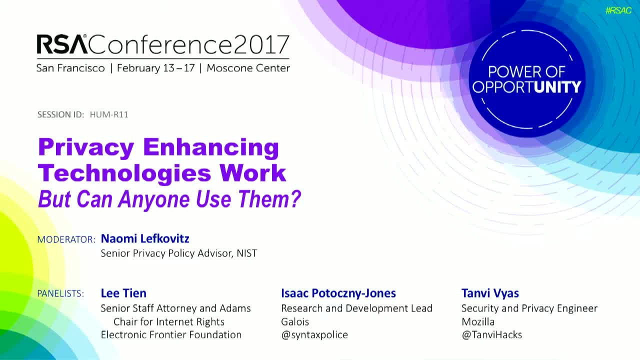 It can be sold to your employer. The thing is is that, since people start out in a world where they believe, as I mentioned before, that a website having a privacy policy means it's not sharing that information, they don't start from a default of thinking that anything they do is going to be collected. 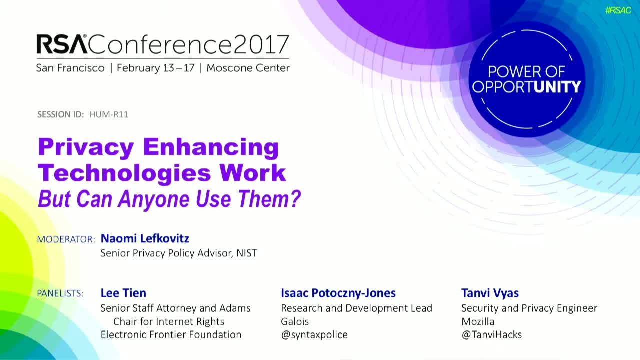 and shared with someone else. They sort of start with this feeling that it's not So. if that's what they believe, then it's actually not crazy for them to sort of walk around giving information. It's not like, well, I'm not going to share this information to websites because they 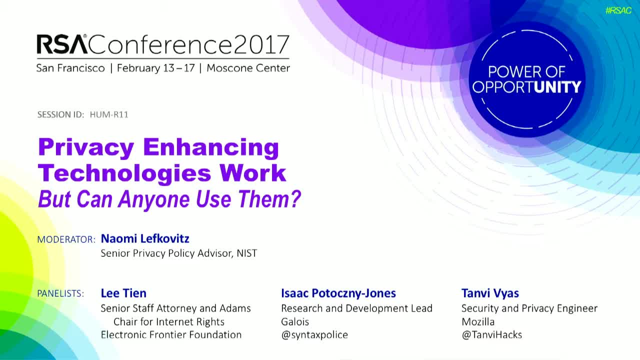 don't think it's going anywhere. They happen to be wrong, But I can't completely fault their behavior, because they're also in this context where the people- the entities that are in the best position to explain to them what is happening to their data- are the very same entities that have the most incentive to collect it without. 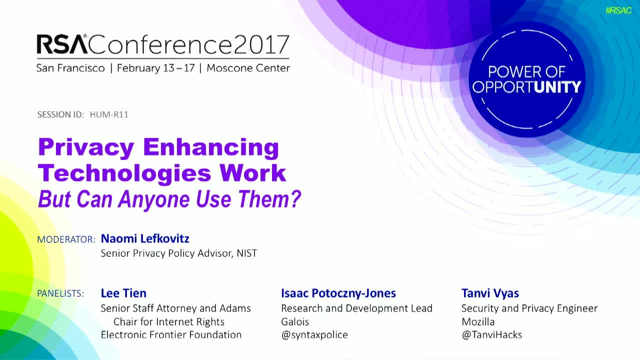 it And to continue that stream. So you can't ask water not to be wet And you can't ask tigers not to be predators, And you can't expect businesses whose models find information to be really useful to A, not collect it and B just go public with everyone and say, yeah, this is what we're. 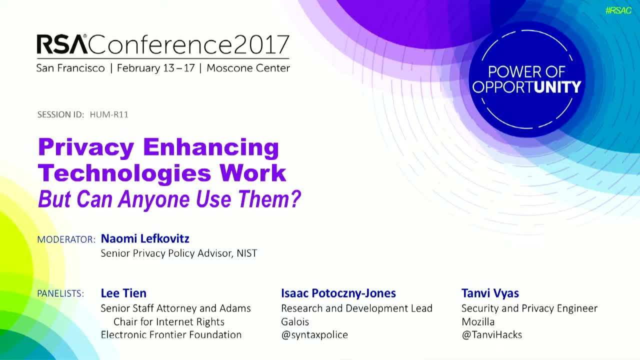 doing. We have to expect that they're not going to and design systems that account for that. So there's a feature in Firefox that I'm creating, called containers, that allows you to separate multiple personas of yourself, So you can have a work tab next to a personal tab, next to a shopping tab next to an airline. 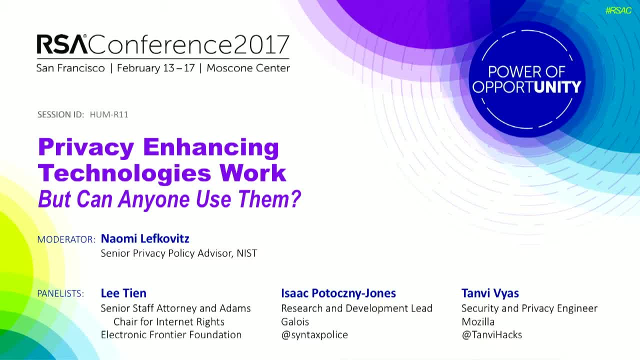 tab And these things like price fixing and data leakage. Okay, So you can see the price, phone number and then you can have a word of mouth in there. So I'm here to just show you what happens. And if you have a lot of resources, you've got like 12 to 15 different tools that you 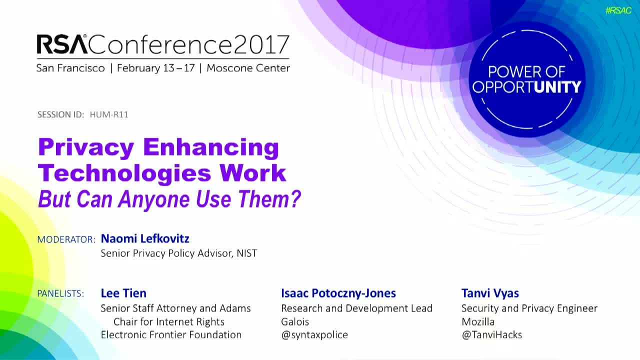 can work with. you can have one here- that's very useful for setting up container- and ask them to do the work, And then, if you have a lot of resources, you can just go to the back end and say, hey, I'm going to share these with you in a minute. 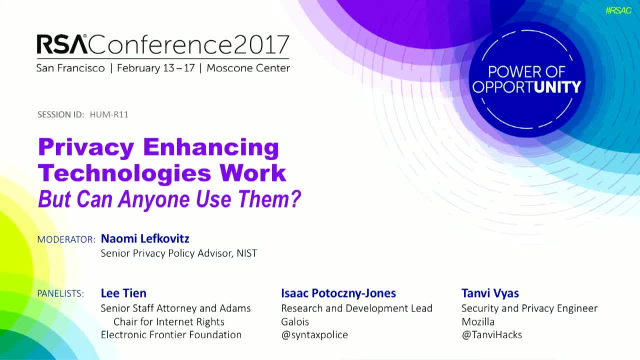 And that way, that's going to come to you on your own. So again, bring the key with you And if you have access, I'm going to play along with it and I'll explain it with you later as well. So I've got a bunch of resources in there. 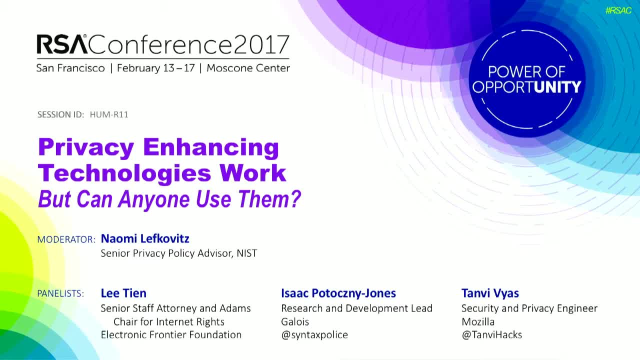 I'm going to just show you how to put those into context to help you develop those in shopping profile. I still get targeted results, which I want in that context, but I don't want them to leak over to work And it preserves my privacy at the same time. 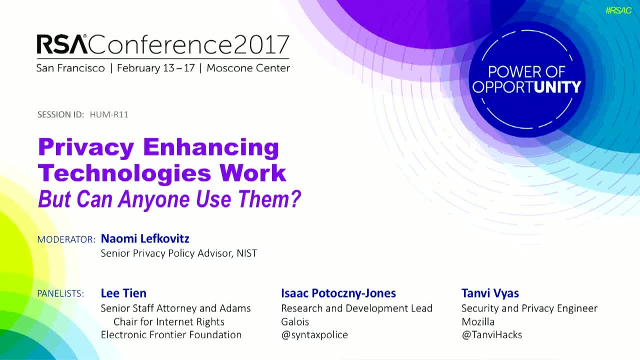 So trying to create tools like that for users that really think about privacy first, but also offer additional benefits, also helps with this. I like that. yeah, Anyone have a last question? Yeah, Jen King from UC Berkeley. Firstly, thank you for citing my research. 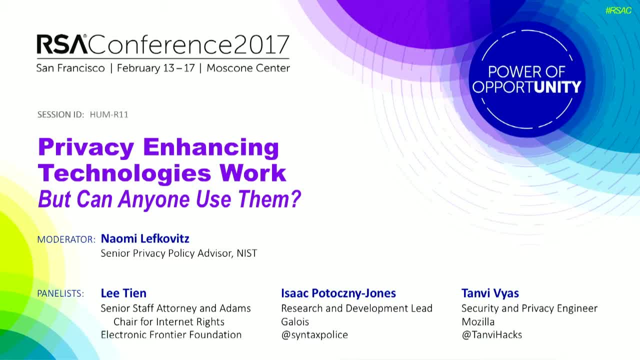 not once, but twice during this panel, even though I don't think you realized it was mine. It's good research, The survey work on privacy policies, awesome, So I wanted to back up a lot of what I've heard. My research area is on human behavior and privacy. 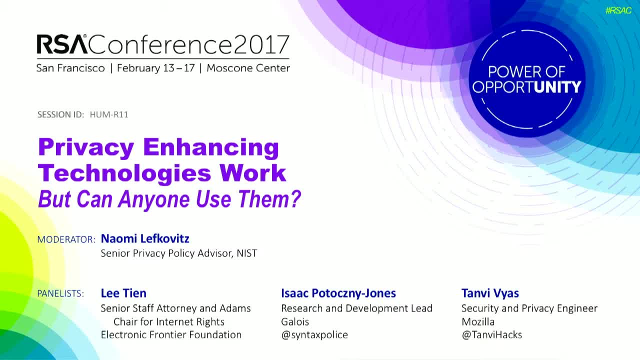 And, yes, users don't know what's going on. they're very confused, and we can go on and on about that topic, But one of the things I think would be helpful in this discussion, which I often find when we talk about PETs- 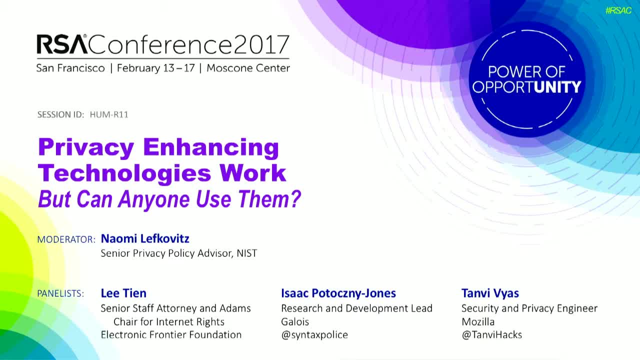 it ends up being a circular argument about why people are blaming the users, because the users don't understand. so why aren't they using these things? what are the incentives? and we just keep going on and on in this circle. So one of the things I think that would be really helpful. 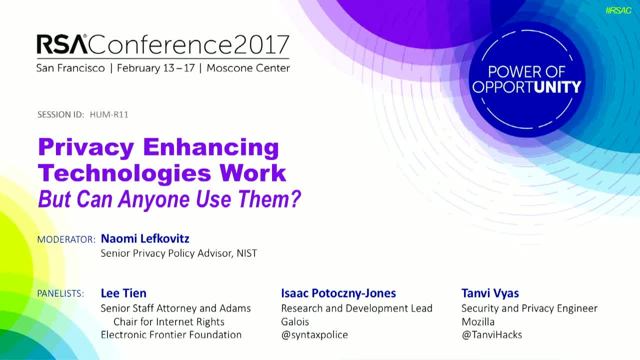 for shifting the discussion is to actually do look at the incentives of the companies, And one of the things I'm doing in my own research is examining why people disclose to companies, And one of the things I think we really don't discuss enough is the fact that it is in these companies' best interest. 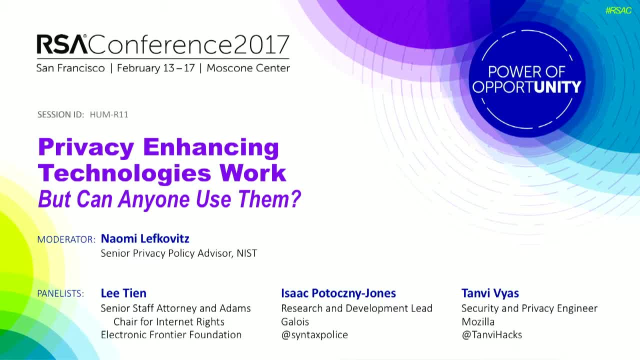 absent the fact that we have legislation really trying to level the playing field to have a trusting relationship with their customers And, to the extent that they can design their products to build for trust, I think is a really important piece of the argument. 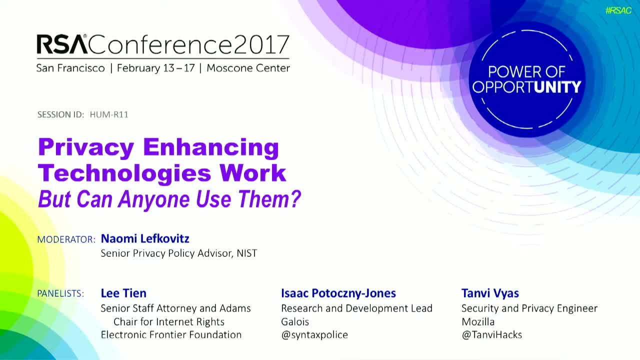 and is very much in the company's self-interest, assuming they actually want to have ongoing relationships with these customers. In the work I'm doing, what I find is that there is a lot of inherent trust people have when they decide to disclose with companies. 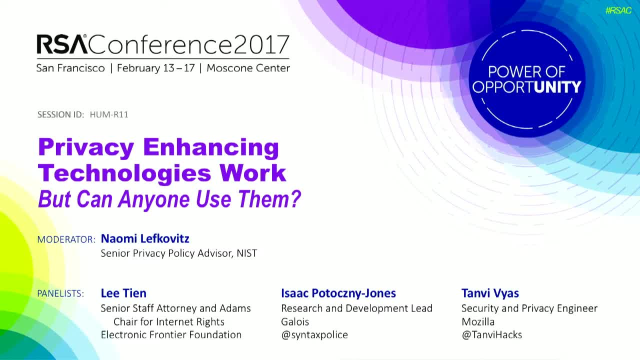 But a lot of that's based on the idea that they think the information is just going to the company and no further. When you start getting into third-party data collection, everything, people throw up their hands and don't like it, even if they don't know what it is. 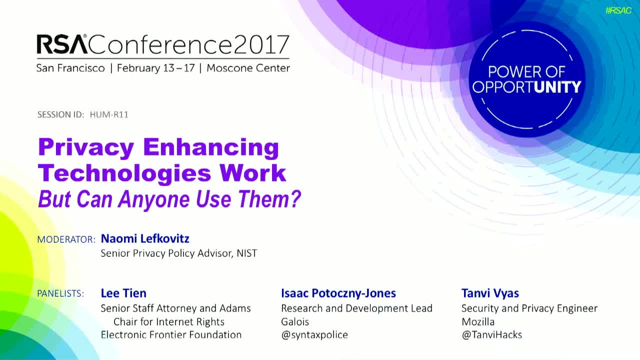 But people are really willing to grant a company quite a bit of leeway as long as they think that it's in the company's best interest to not sell information, to not be caught doing something wrong. So there are levers in the marketplace.